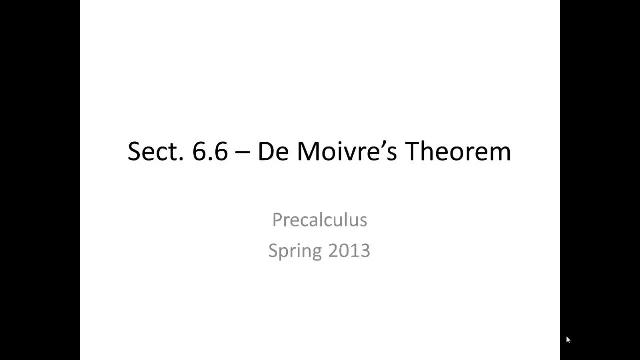 Now, of course, you might think, well, there's one easy way to make sure that prediction comes true, and maybe he did that. But then maybe this whole story is complete and utter hogwash, which is probably the case anyway. But it's a fun story anyway. 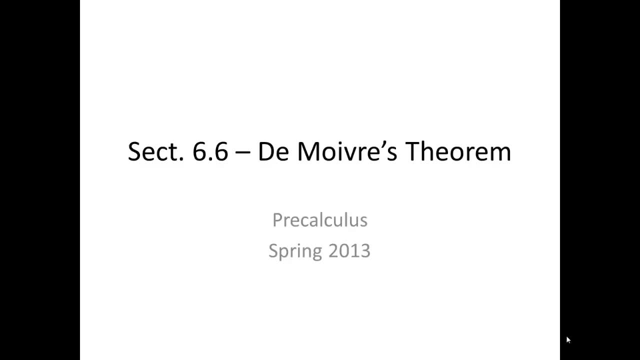 So Dumois: We're going to learn about Dumois' Theorem in section 6-6.. Now Dumois' Theorem. we got a lot of prep work before we can actually get to Dumois' Theorem. It's actually the last couple of slides right at the end of the presentation is going to be Dumois' Theorem. 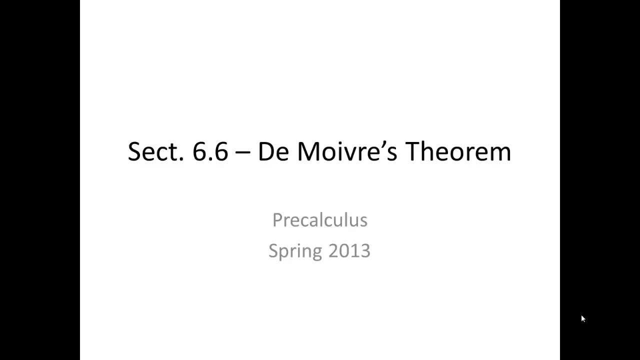 Everything else, though, leads us up to Dumois' Theorem, So let's go ahead and start at the beginning so that we can get to the end, And the beginning is the complex number plane. Let's remember that complex numbers are any number of the form a plus bi, where i is not the unit vector i, but the imaginary number i, square root of negative 1.. 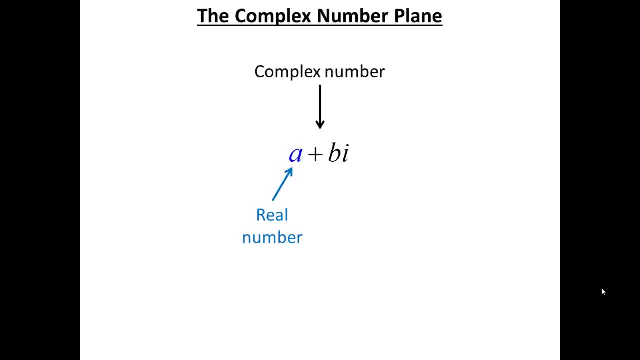 So a represents minus my real number and bi represents my imaginary number. So if I take a real number and an imaginary number, put them together I have a complex number. Now we can plot a complex number on a complex number plane and we get the complex number plane by starting with a real number line. 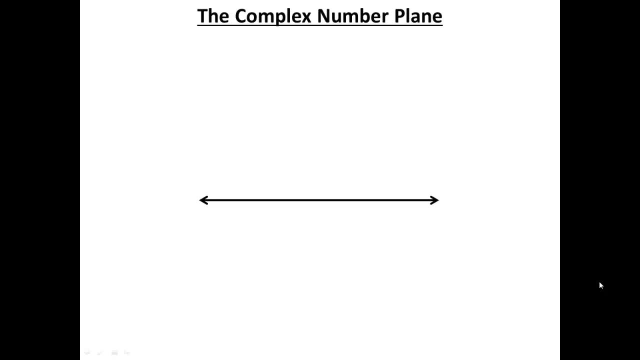 So imagine if I'd said: plot the number 4 on a number line. well then I could just go on the number line, define somewhere to be 0, and then just plot 1,, 2,, 3,, 4.. 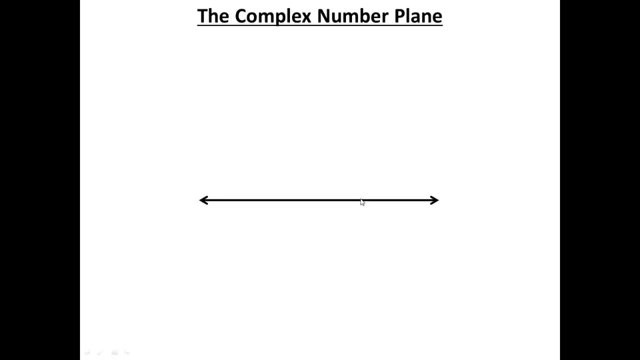 and that would be number 4 on the real number line. The problem is, if I said plot the number 4i on that number line, it wouldn't make any sense because that's a real number line. There are no imaginary numbers on the real number line because the imaginary number line is actually perpendicular to the real number line. 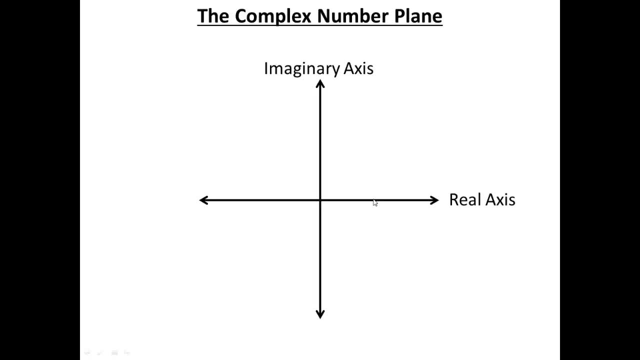 So if I take the two number lines for real numbers and imaginary numbers and put them together, we have a number plane, referred to as the complex number plane, where the x-axis is now the real axis. so we'll plot real numbers along the originally called the x-axis and then the y-axis is your imaginary axis. 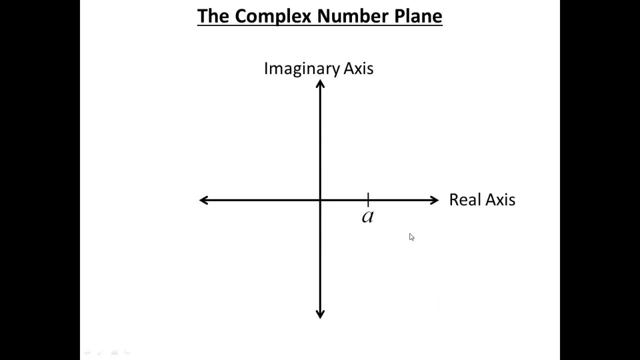 So if I give you a plus bi, well, a is on the real axis, b is on the imaginary axis. so the number a plus bi can be plotted just like a coordinate is on the xy coordinate plane, where a is your x and b is your y. 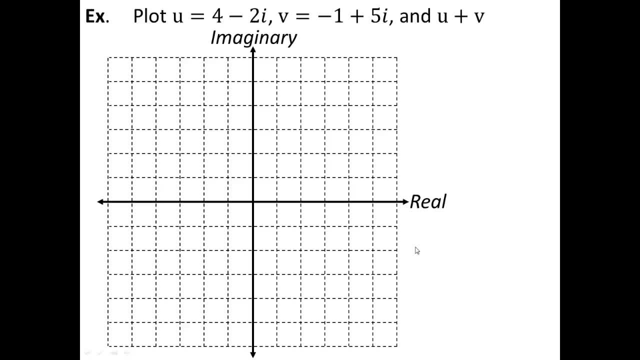 So let's go ahead and take a moment. This is a coordinate plane. Let's go ahead and plot 4 minus 2i, negative 1 plus 5i, and then let's plot the sum of those two complex numbers. 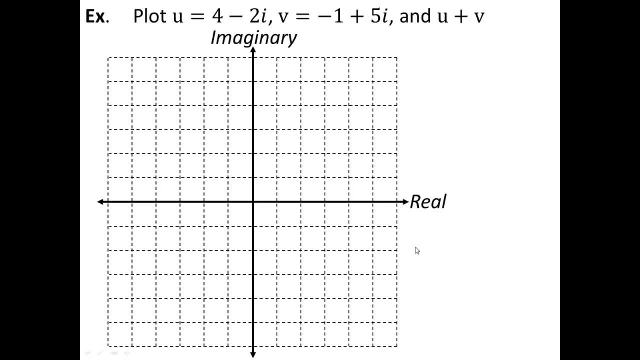 I'll give you a second to try it out on your own Hit play when you're ready. Alright, so 4 minus 2i. well, if it's 4 on the real axis, 1, 2,, 3, 4, down 2, that would be right here. 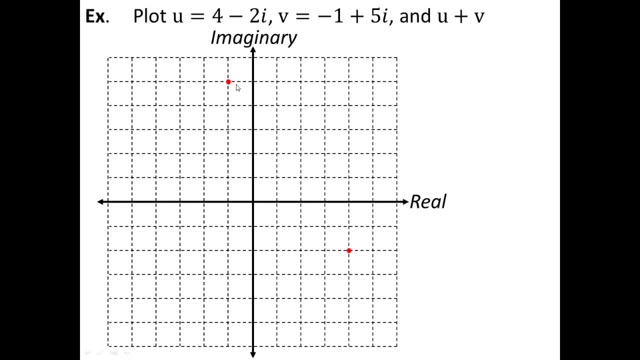 And then negative 1 plus 5i. so negative 1, up 5,. that's going to be up here. Now, if I want to plot the sum of those two complex numbers, I'm going to do this. If I wanted to plot u plus v, well, that's just a matter of taking the complex number u, the complex number v and adding them together. 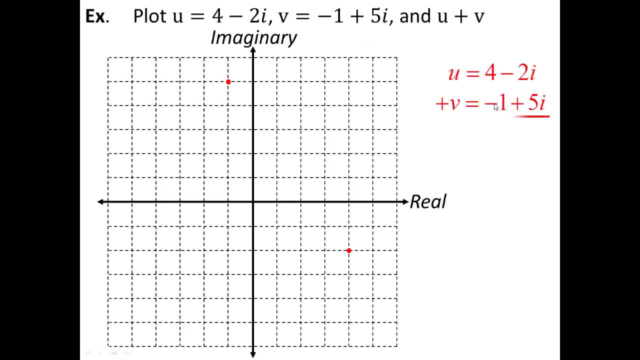 So to add them together, just combine like terms. So 4 and negative 1 would give us positive 3, and negative 2 plus 5i would also give us positive 3.. So u plus v is really just 3 plus 3i, which would be right here. 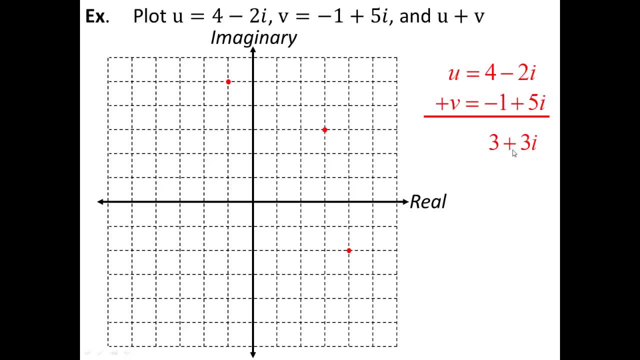 Now hopefully you're kind of making connection here- We're at the end of chapter 6.. This is actually very similar to what we started with in chapter 6 with vectors. If I thought of 4 minus 2i, instead of that being the complex number 4 minus 2i, if I thought of that as the vector, let's say 4i, vector i, not complex number i, 4i minus 2j. 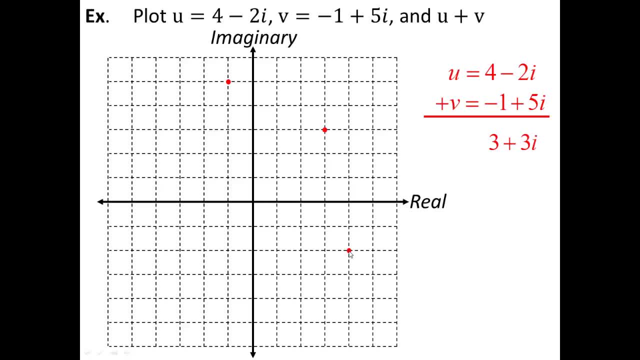 well then that would be a vector that's going 4 to the right and 2 down right at the same spot. the complex number is, but it would be a vector. Same thing if I had vector negative 1 plus negative 2j. 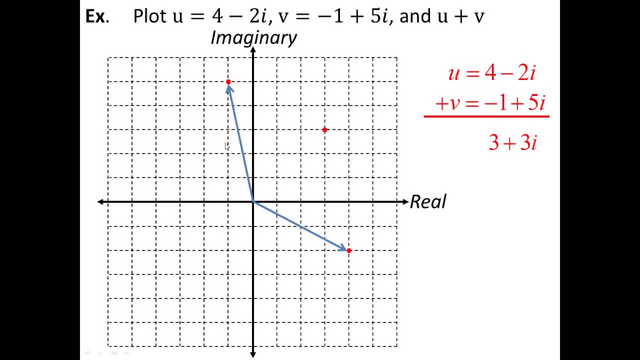 Negative 1i plus 5j- that would be this vector right here- And to add two vectors together to get u plus v, in other words the resultant vector, instead of doing it arithmetically like I did over here. 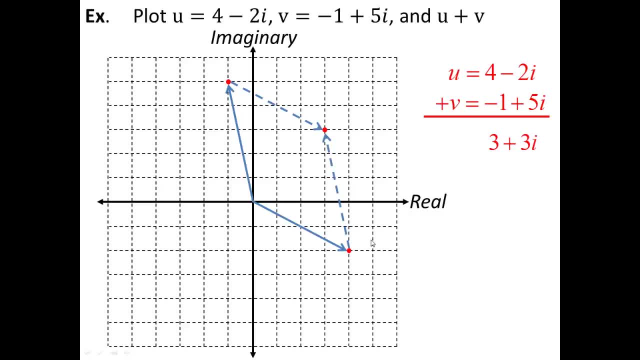 I could have just taken this vector and this vector and built a parallelogram and drawn the resultant vector connecting them. So as we go through this section on complex numbers, we hopefully will see that really this is not new information, This is old information. 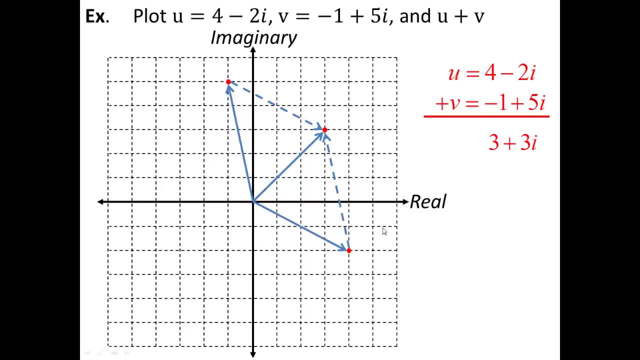 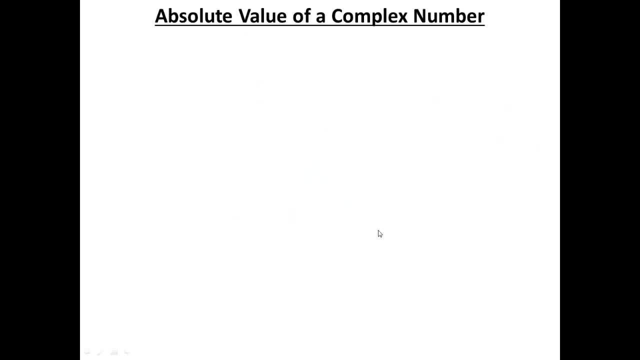 This is just vectors, polar functions, parametric functions repackaged as complex numbers. It's all the same stuff, it's just under a different name. Alright, let's find the absolute value of a complex number. We found the absolute value of a vector simply by applying the Pythagorean Theorem: a squared plus b squared. 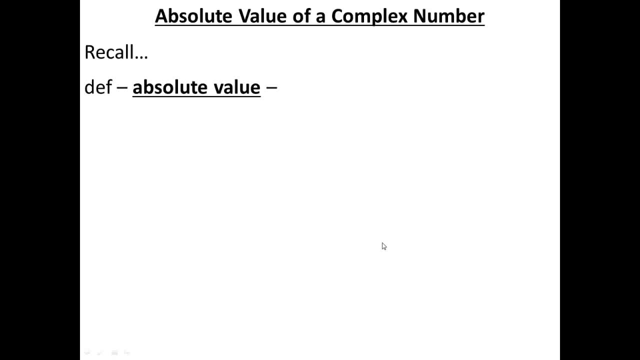 Now let's find the absolute value of a complex number. And the way we're going to find the absolute value of a complex number is if we recall that absolute value just means distance from 0. If I think about the complex number a plus b, i let's just call it complex number z. 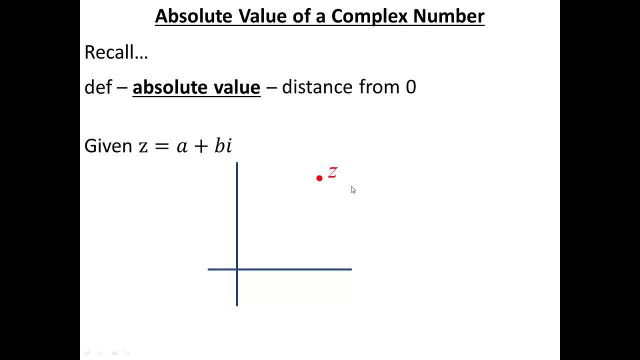 If I plotted a plus b, i, that would be- let's say it was right here, so that this would be a, this would be b, and then the direct distance from the origin would be this distance right here. Call it the absolute value of z. 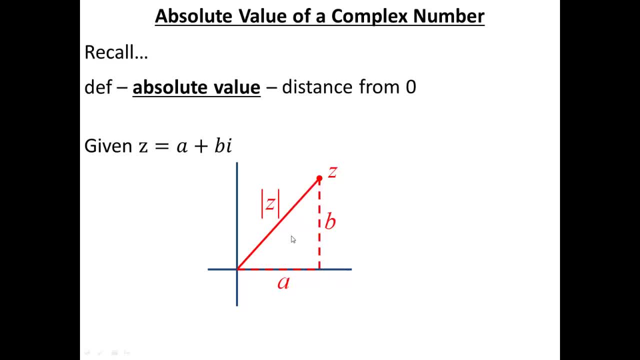 In other words, it's the exact same thing. Absolute value of a binomial, whether that binomial be a vector, an a and a b component for a vector or an a and a b for a complex number, Is still going to be the square root of a squared plus b squared. 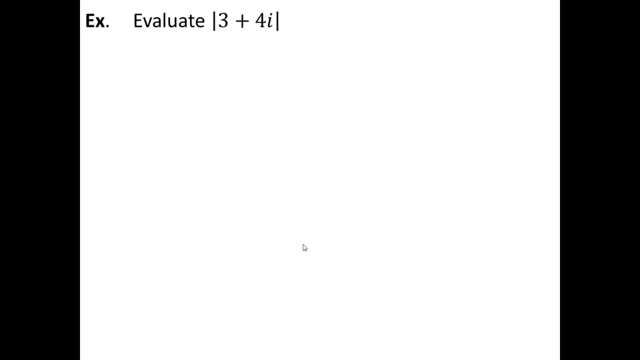 Alright, go ahead and evaluate the absolute value of 3 plus 4i. Hit play when you're ready. Alright, absolute value of 3 plus 4i. that's just the Pythagorean Theorem, with 3 and 4 being your a and your b value. 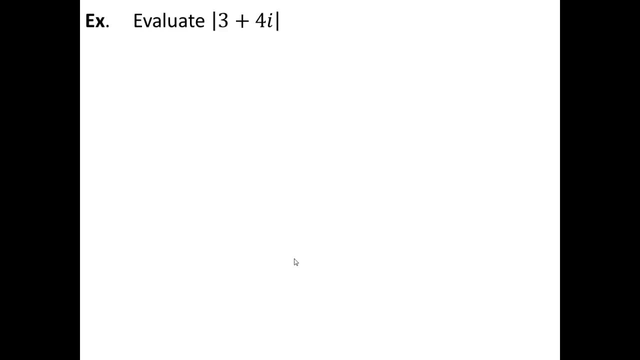 Hopefully you didn't have to do any work whatsoever, because 3,, 4,, 5.. If a and b are 3, or a and b are 3 and 4,, then the c value must be 5.. I could completely and utterly waste my time by drawing a picture. 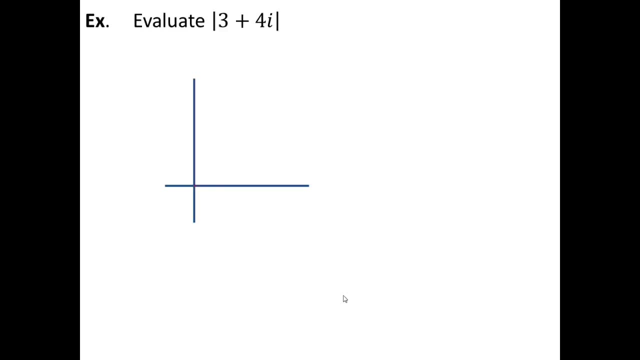 Hopefully you don't ever draw a picture for something like this, but I just wanted to illustrate what it would look like. One side is 3,, the other side is 4, we're looking for the hypotenuse Again: 3,, 4,, 5, I know the hypotenuse is 5.. 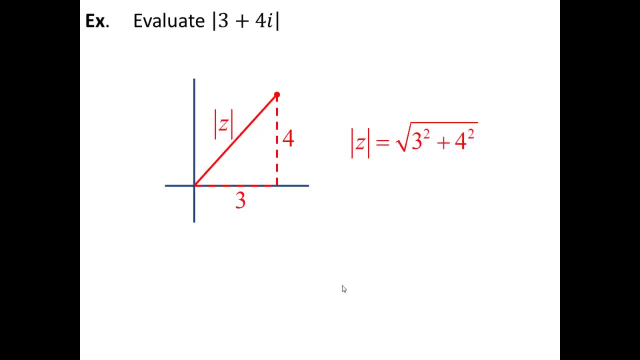 I can arithmetically prove it by doing the Pythagorean Theorem: 3 squared is 9,, 4 squared is 16, the hypotenuse is 5.. Alright, let's do it again. Hit play when you're ready. 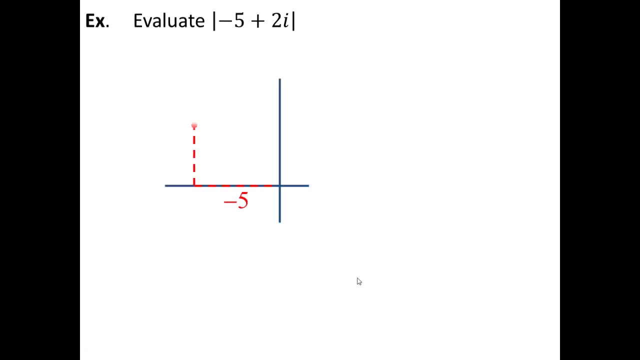 Alright, once again I could waste time by drawing it, or I could just do the Pythagorean Theorem: Negative: 5 squared is 25,, 2 squared is 4, 25 and 4 is root 29.. Moving on. 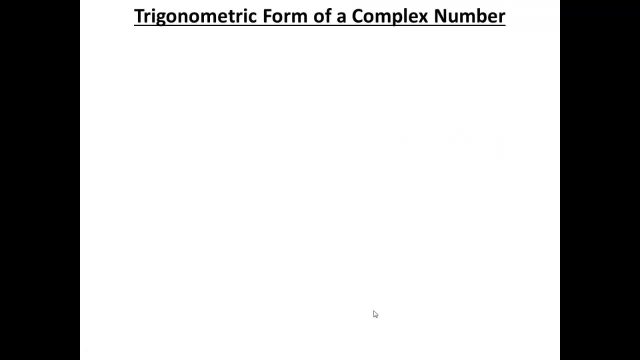 Alright, trigonometric form of a complex number. Now the form that we've been writing it in so far is actually referred to as the standard form. a plus bi is the standard form of a complex number. Anytime you're asked to write a complex number in standard form, that is a plus bi. 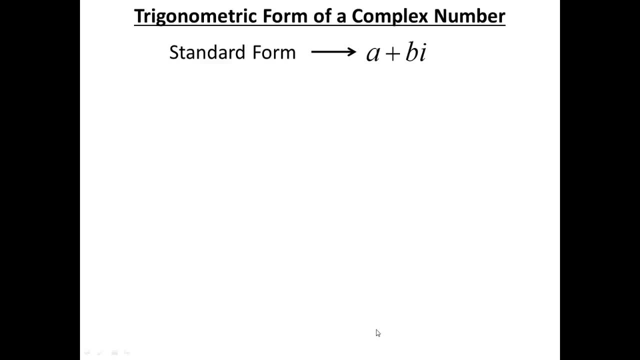 Now, trigonometric form obviously is going to have some trigonometry involved, So trigonometry has to do with right triangles. So let's think about what a plus bi looked like when I plotted it. Now, a and b were the x and y components. 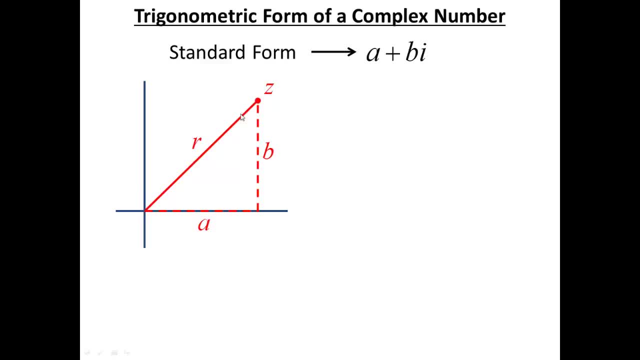 and then this was the absolute value of the complex number. But in order to simplify things, let's just go back to that polar notation and use r to represent the radius of that complex number. So we know that r is just the square root of a squared, plus b squared. 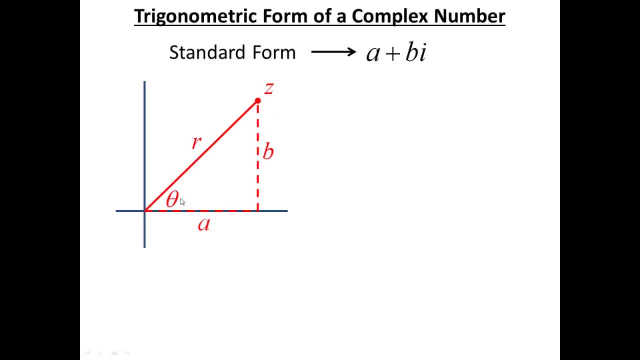 And we also know that we can throw in a theta right here so that we can define what a and b actually are. So a, if you think about it, shouldn't have to think about it too long, because we've been using these same formulas over and, over and over again. 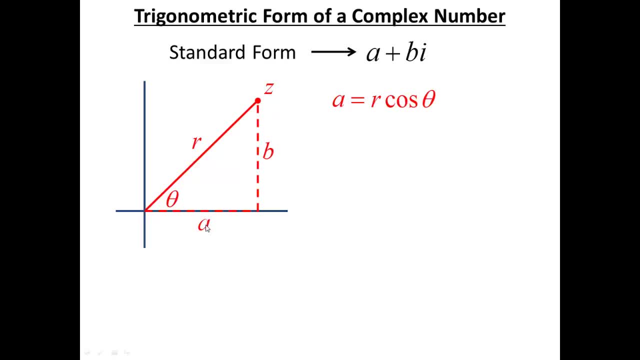 Well, a is the x component. Therefore it must be r cosine theta, because a over r is cosine. So if I move the r to the other side, then I get a equals r cosine theta, Just like in polar it's x equals r cosine theta. 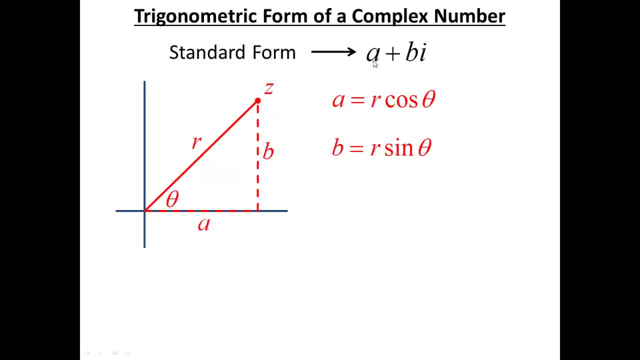 And for that matter b would have to be r squared. So if I replace a with r cosine theta and b with r sine theta, then I get r cosine theta plus r sine theta i. But since both of these have an r, we just factor it out and call it the trig form. 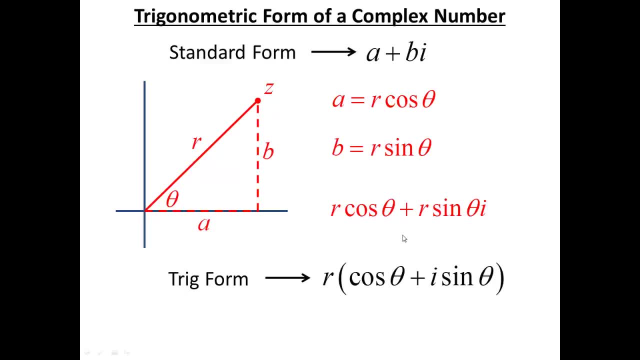 So the trig form of a complex number is just r, parenthesis- cosine theta plus i sine theta. Now notice I also moved the i to the front. It doesn't matter where you put the i, If it's i times sine or sine times i, it's still the same thing. 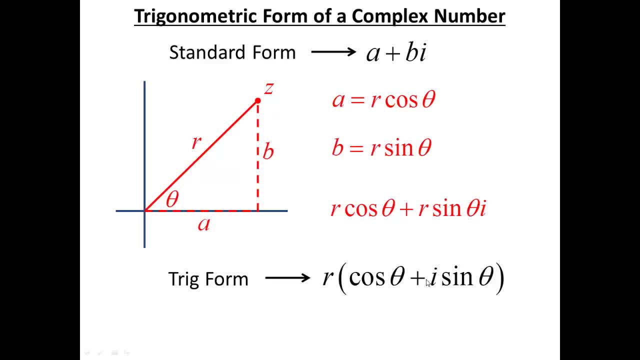 because it's the same thing: Multiplication and multiplication can be done in either order, But it's common to put the i in front in order to avoid confusion. Right here it's possibly ambiguous. Is that i part of the angle or is that i being multiplied by the entire sine ratio? 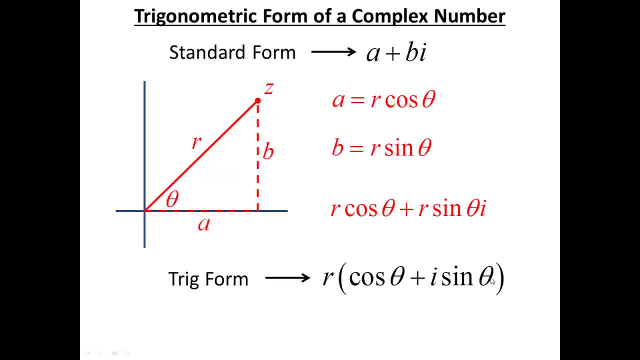 Versus. on this one, it's perfectly clear. i is not part of the angle. i is being multiplied by the sine ratio, So let's just put the i up front in order to be perfectly clear. Now, just for kicks, I'm going to go ahead and tell you. 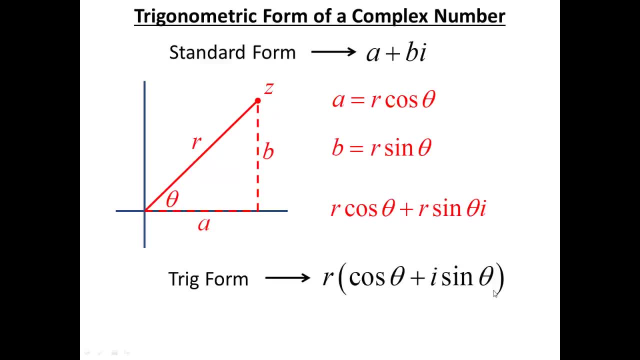 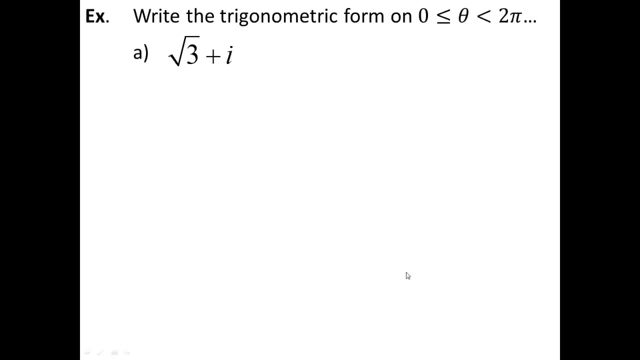 sometimes this is referred to as the trig form. It's also commonly referred to as the polar form of the number And the polar form because of that same basic notation. a polar coordinate is r, theta And in trig form, those are the two pieces of information we need to know: r and theta. 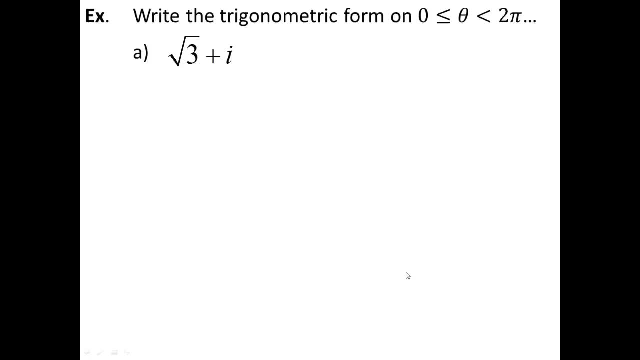 Alright, so let's practice a little bit. Let's write this standard form of a complex number in trig form. Notice: it says on the interval 0 to 2 pi. So that tells us that the angle has to be a radian, not a degree. 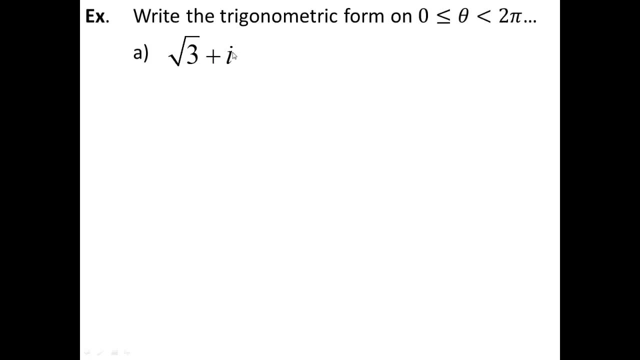 So we're going to start with root 3 plus i. Now keep in mind that there is an imaginary 1 in front of that i right here. So that means our a value is root 3, our b value is 1.. So as we go through this process, the i is not the b value. 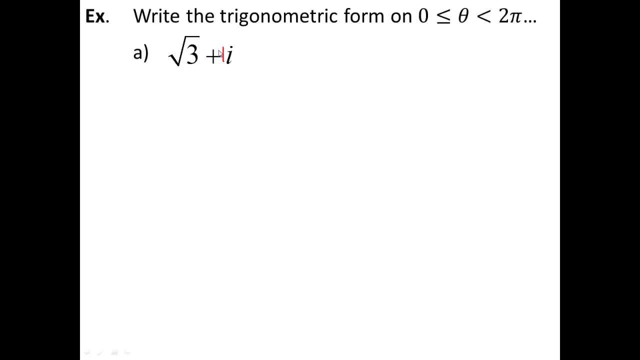 The i is the number that signifies, which is the b value. So the fact that the i is not part of the root 3 means that the 1 is the b value, the a value is root 3.. It's just like: y equals mx plus b. 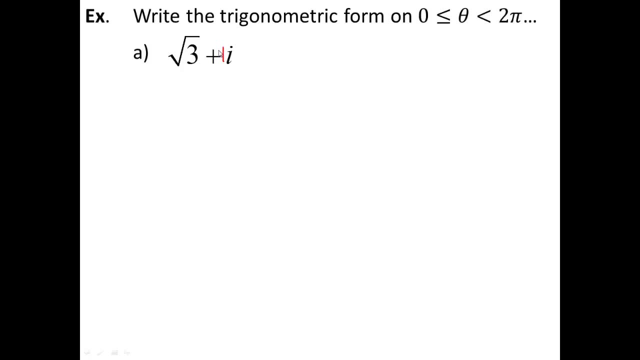 If I give you, y equals 2x plus 5, the slope is not 2x. the slope is 2. Because it's the number in front of the x and it's not 5 because there's no x attached to the 5.. 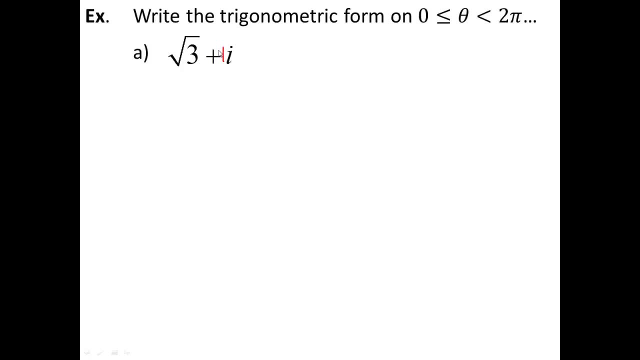 I see this all the time of people trying to throw in the i value as part of the b. No, the b value is in front of the i, It's not the i itself. So to write it in trig form, first thing I'm going to do is I'm going to figure out the r. 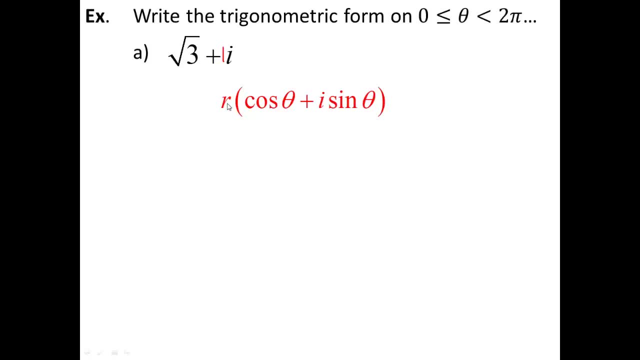 by using my handy dandy Pythagorean theorem: a squared plus b squared, So it's going to be root 3 squared, Which is 3.. And then 1 squared, which is 1.. Add it together, I get root 4, which is 2.. 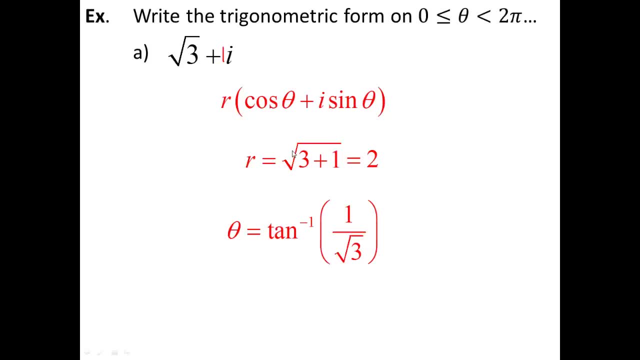 So r is 2.. The only other thing I need to figure out is the angle. And to figure out direction angle we just go back to that same standard formula. we've been using the inverse tangent rule: of b over a, 1 over root 3.. 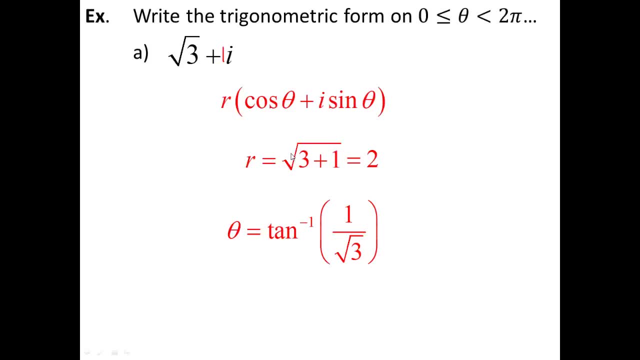 Now, this is a unit circle value. I shouldn't need any calculator for this Inverse tangent of 1 over root 3.. Well, tangent is really sine over cosine. So the question is: when is sine equal to 1?? When is cosine equal to 1?? 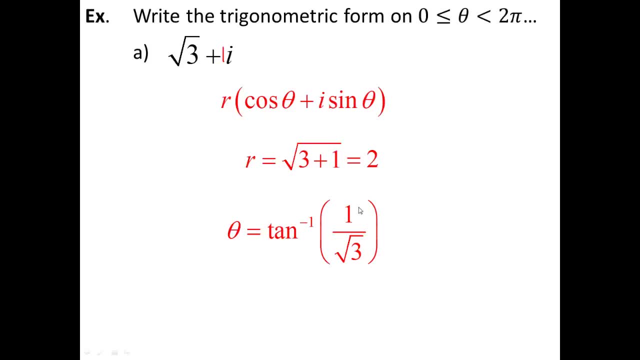 When is cosine equal to root 3?? But what we often do is we realize that's not really 1. That's actually 1 half And that's root 3 over 2.. So when is sine equal to 1 half? 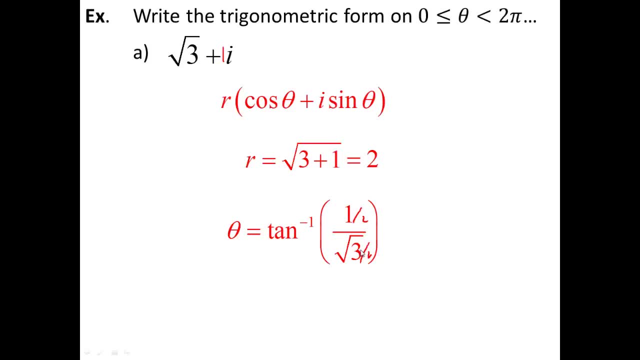 When is cosine equal to root 3 over 2?? Well, that's at pi over 6.. And I'm also going to make sure I pay attention to the quadrant Root 3 and positive 1. Positive- positive means I'm in the first quadrant. 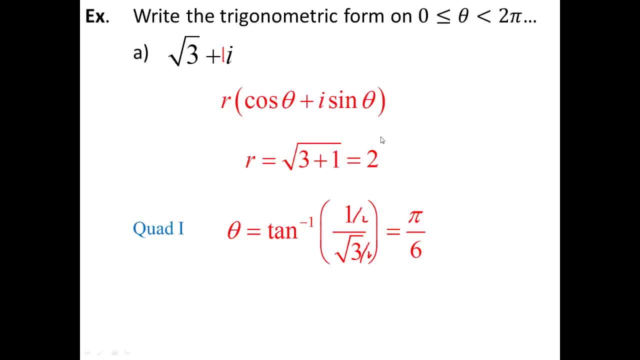 So pi over 6 is going to be my final answer on that. So r is 2.. Theta is pi over 6.. So I can write my trig form. I can write my trig form just by plugging in the numbers 2, cosine of pi over 6 plus i sine of pi over 6.. 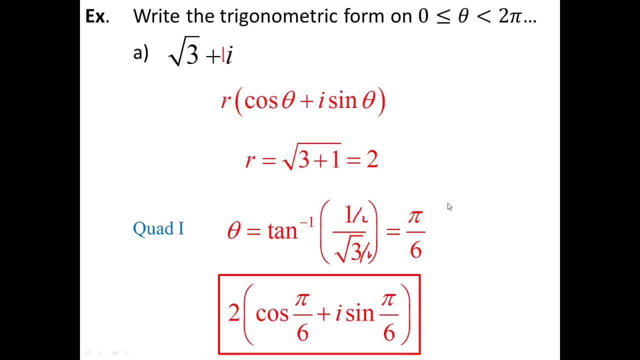 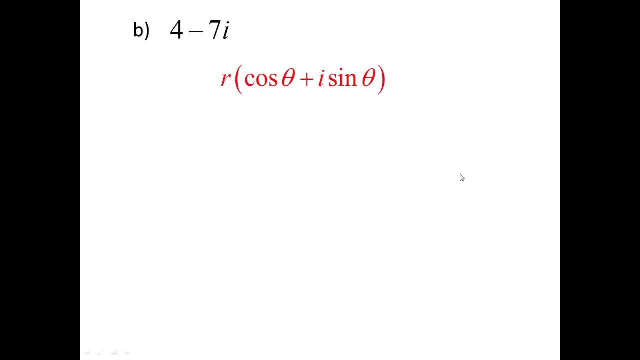 Final answer: All right, So we see how easy that was. Let's try it on our own. 4 minus 7i. Give it a try, All right, So 4 minus 7i. We'll start by finding the r value by doing the Pythagorean theorem. 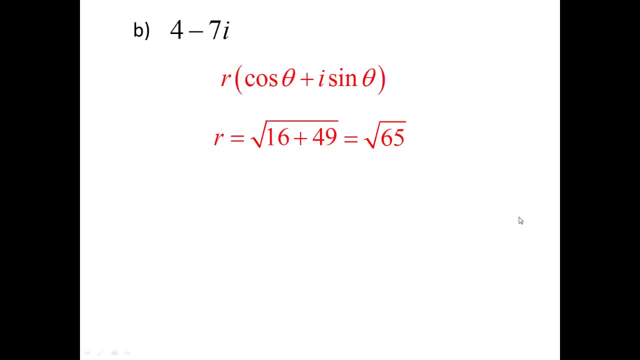 4 squared and 7 squared is going to be 16 and 49.. Add it together, We got 65.. We're going to leave it as root: 65.. Now, to get the angle, I'll do the inverse tangent of negative 7 over 4.. 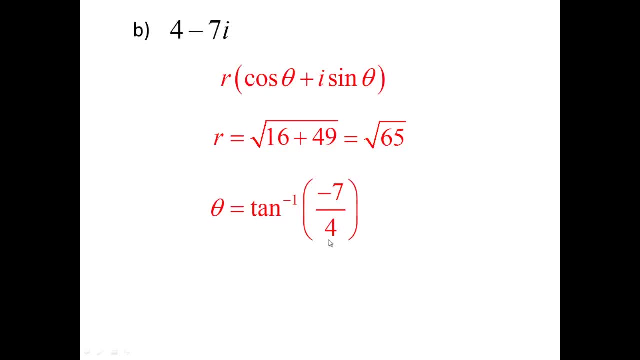 And hopefully you pretty quickly realize this is not a unit circle value. So I'm going to want to get my calculator out. Also, remember that that calculator needs to be in radians And since I'm going to be using my calculator, I may need to make some adjustments with the calculator. 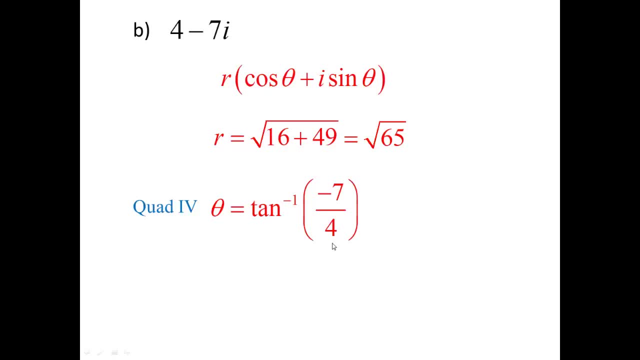 I am in the 4 negative 7. So I'm in the fourth quadrant, And in the fourth quadrant I would think normally of a 360-degree adjustment, But since I am doing this in radians, it's going to be a 2pi adjustment. 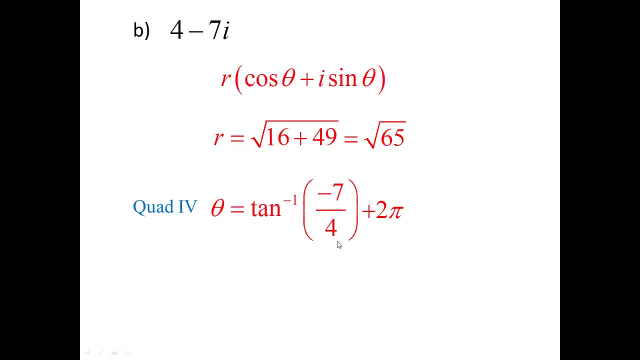 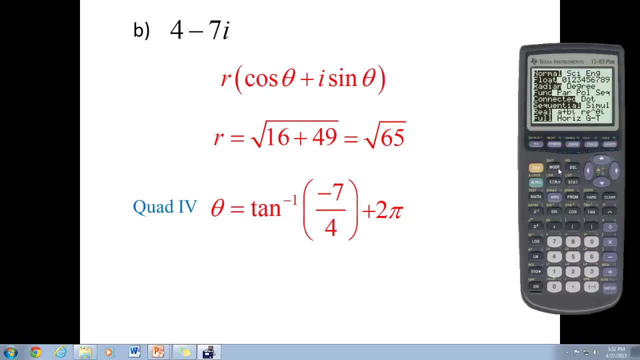 So I will add 2pi as part of the process, All right, And then I will pull up my calculator. Let's go ahead and clear that out. Make sure I am in radian mode, which I am, All right. So I'll go ahead and type that in. 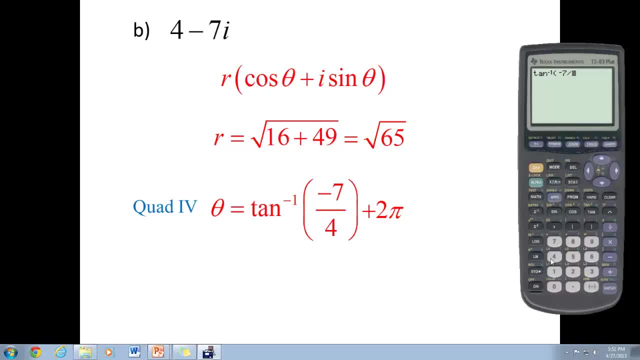 Second tangent of negative: 7 over 4.. Close that parenthesis Plus 2pi And I get 5.231.. So my direction angle is 5.231.. And my radius is root 65. So 5.231.. 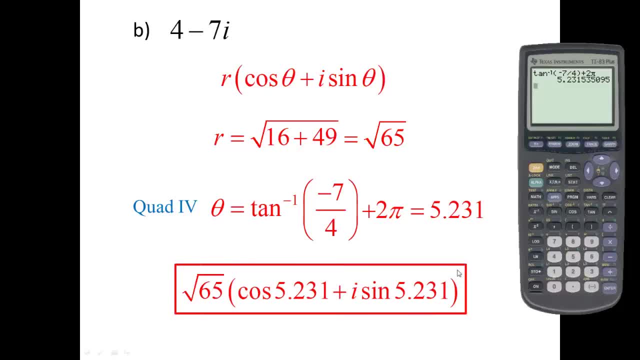 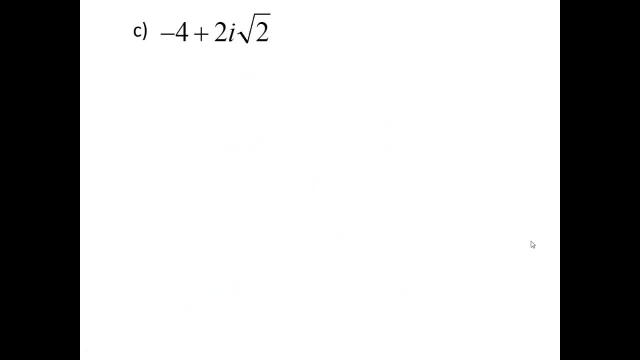 We can put it together in my trig form: Root: 65 cosine of 5.231 plus i sine of 5.231.. All right, Here's a new one. Go ahead and try this one on your own. Hit play when you're ready. 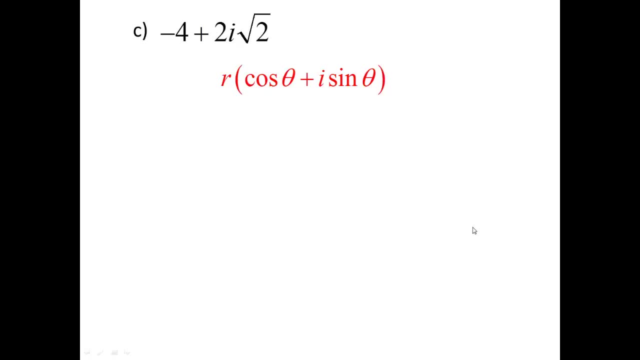 All right, We will start with our trig form. I've got to figure out the r value by doing the staggering theorem: 4 squared is 16.. And then 2 root 2 squared: 2 squared is 4.. Root 2 squared is 2.. 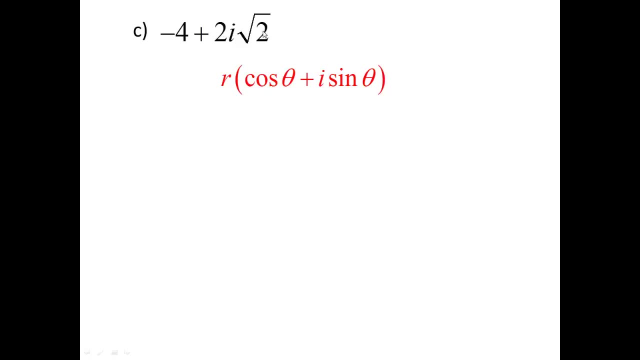 4 times 2 would be 8.. So that would be 16 plus 8. Or root 24.. So r is root 24.. Let's get the direction angle by doing inverse tangent of 2 root 2 over negative 4.. 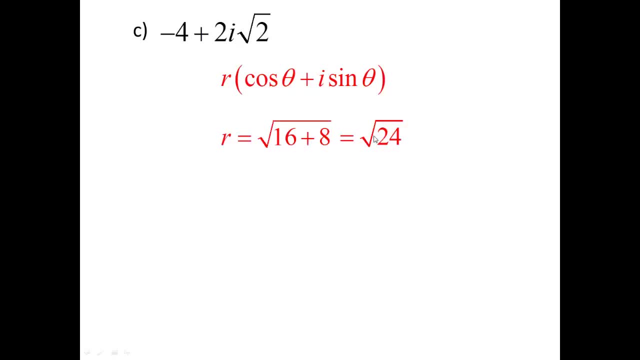 Now, before I decide whether I need my calculator or not, we're going to look at this number on the inside: 2 root 2 over negative 4.. And I really want to make sure that I'm doing it correctly, So I'm going to go ahead and do that. 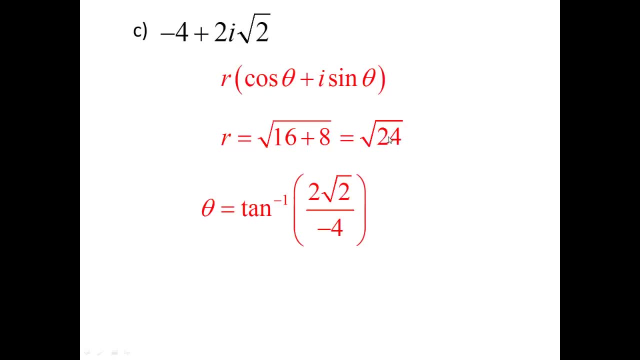 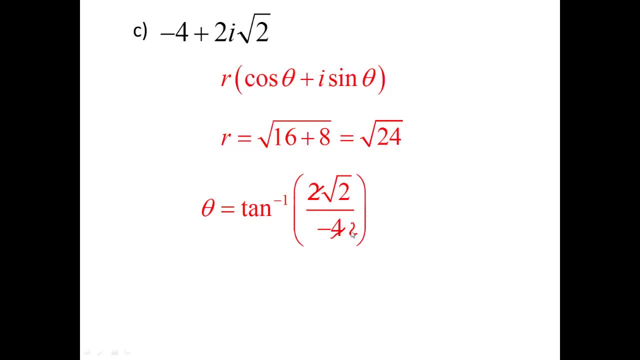 And then I realize: well, it's a unit circle angle for sine and cosine, but not for tangent. Tangent is sine over cosine. If I get root 2 over 2, which is at pi over 4, the tangent ratio is actually 1 overikat. 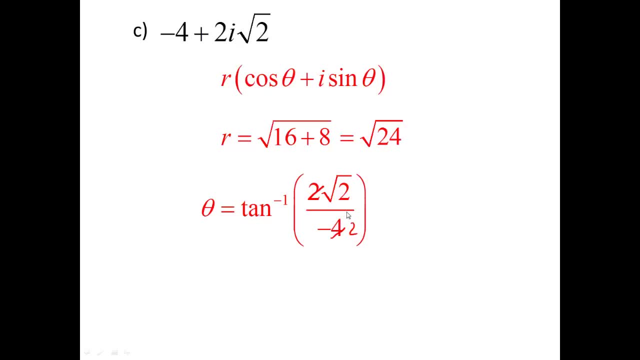 squared 1, not root 2 over 2. so even though it's looks like a unit circle angle, it is in fact not so. what I'll go ahead and do is I'll go ahead and realize that this is in the second quadrant- negative 4, positive 2, root 2, second quadrant, which means my adjustment is not 180 degrees. but 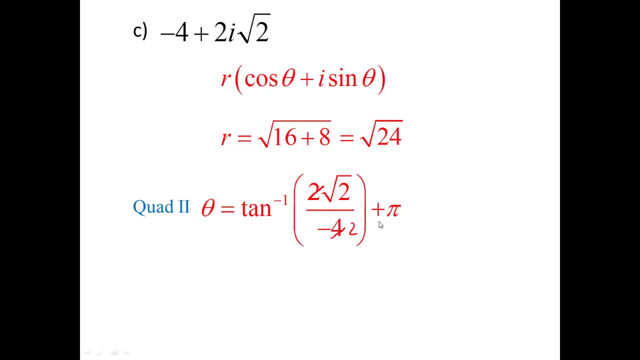 pi, because we are in radian mode, and then I'll pull my calculator back out, type that in and I'm going to get 2.526. so I get 2.526 for the angle root, 24 for the radius and I have my final answer. 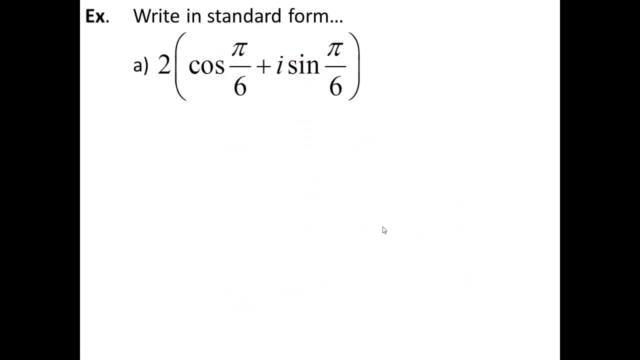 all right now. if we can go in one direction, we ought to be able to go in the reverse direction. so this time I'm giving you the trig form and I want you to simplify it back to standard form, and simplifying back to standard form is really just that. just simplify it. evaluate what you have. 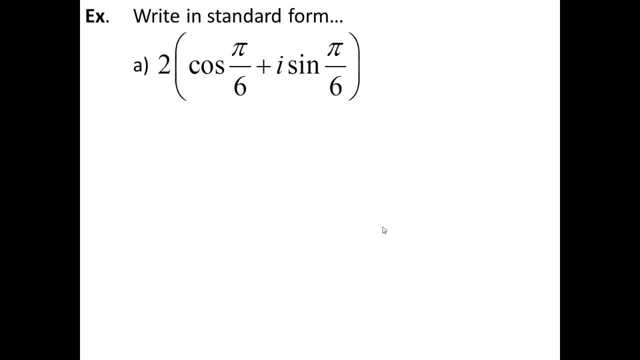 cleaned it up and it will magically be in standard form. you so: cosine of pi over 6- well, that's going to be root 3 over 2. sine of pi over 6, that's going to be one half. then simply distribute the 2 across, so 2 times this fraction is going to cancel out. 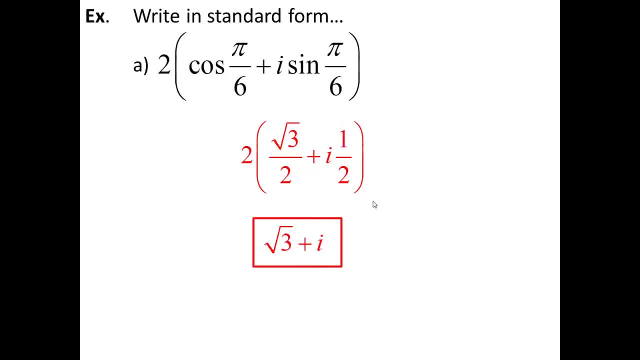 that 2, 2 times this fraction is going to cancel out that 2 and I have root 3 plus i, which actually, if we think back, that was the example that I gave you, the first example that I gave you, for converting to trig form. so we realize that once I've converted to, converted root 3 plus i into trig form, 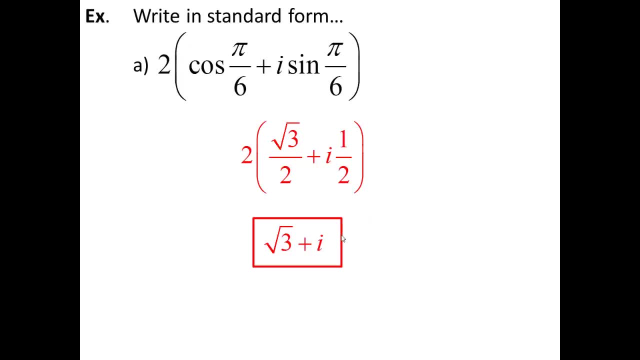 so, which is sign that this is the current way that we're going to go. so if we think back to the original formula, I'm going to have to worry about if I remember trying to change this again. just to check my answer. all I really have to do is resimplify it back to standard form, if I get. 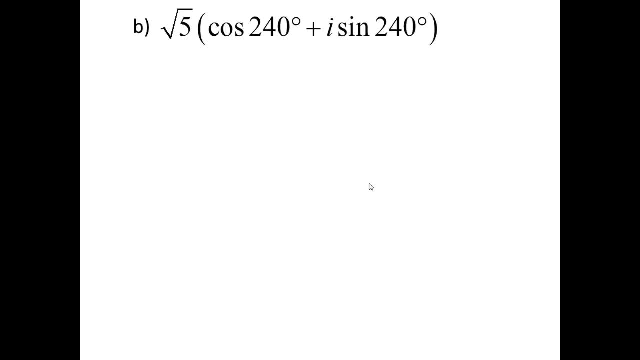 back to what I started with then I know I was right. all right, here's one for you to try. on your own notice, I switched back to degrees, just for fun. hit, play when you're ready. all right, cosine of instead. 240 is a 60 degree reference angle, if I think it back to 180. so 60 degrees is pi over 3. 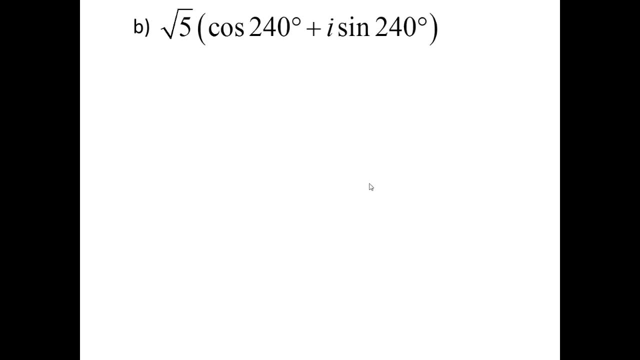 so we are in the third quadrant. so this is going to be 4 pi over 3 as a radian. so cosine of any pi over 3 angle is always going to be one half. third quadrant is going to be negative one half. so I'll have negative one half for the cosine and negative root 3 over 2 for the sine, if I 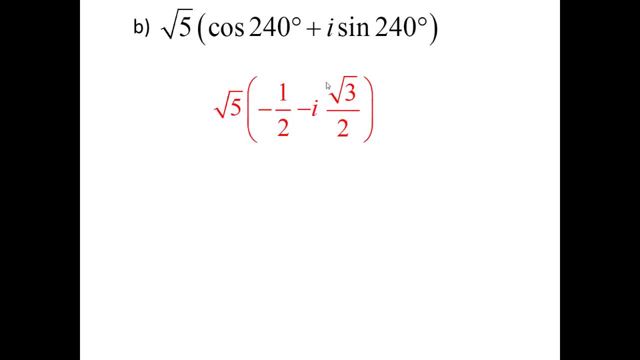 distribute through the root 5. root 5 times 1 is just root 5. root 5 times root 3 is root 15. final answer: alright, so now we know how to write complex numbers in both standard and trigonometric form. now let's talk about multiplying and dividing complex numbers. now, given complex numbers in 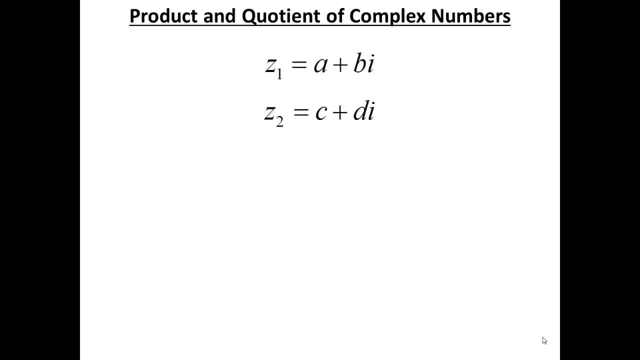 standard form. we already know how to multiply and divide with this. we did this much earlier in the course, as well as in algebra 2. imagine I were multiplying and dividing and dividing and multiplying these two complex numbers together- well, that's really just foiling them out. 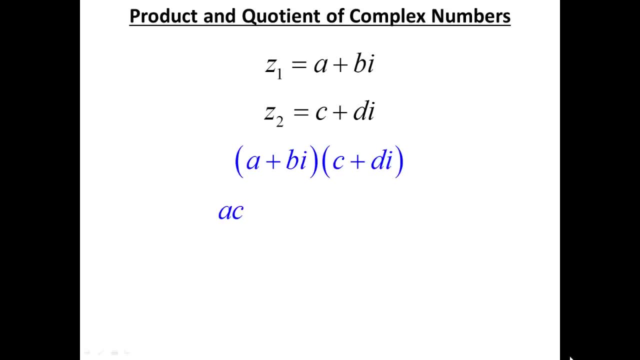 a plus b i and c plus d i. if I were to foil them out- a c plus a d, i plus b c, i plus b i, i'm sorry, b d i squared. well, i squared, of course, is just negative 1, so that would just be minus b d. so if 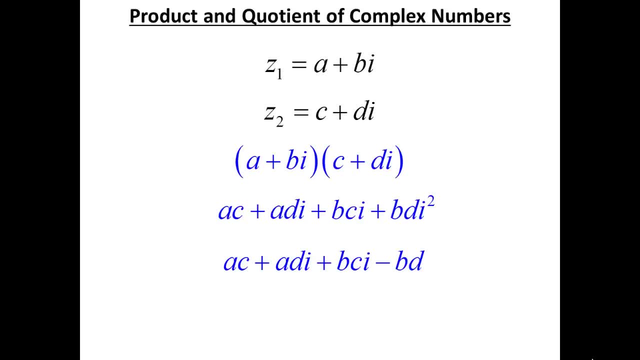 I were to foil it out pretty straightforward, pretty easy, not too bad. but I could also do this in trig form. there's no reason. like if I give you a number of times, I could do it in trig form. like if I give you a number of times, I could do it in trig form, like if I give you a number of times. 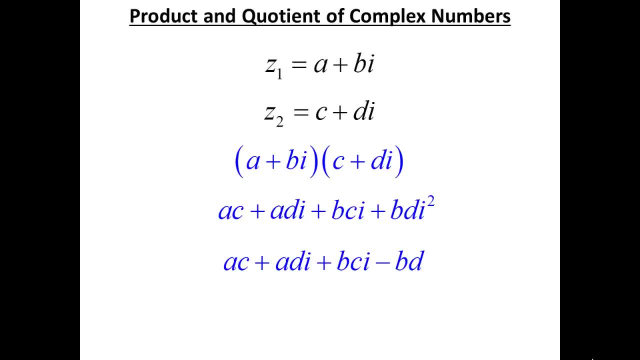 a complex number in trig form, there's no reason I have to waste the time getting it back into standard form before I multiply it together. I can multiply it together straight from trig form as long as I realize a certain shortcut. So let's look at the same complex numbers now in trig form. 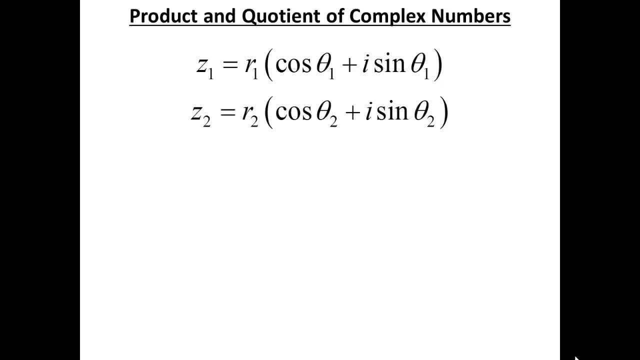 so z1 is r1 cosine theta 1 plus i sine 1 sine theta 1, and then z2: everything's just labeled with 2.. Now, of course, I could simplify these to standard form and then multiply it through, or I can just multiply it through right now. Now I'm going to do this the long way first, and then we'll. 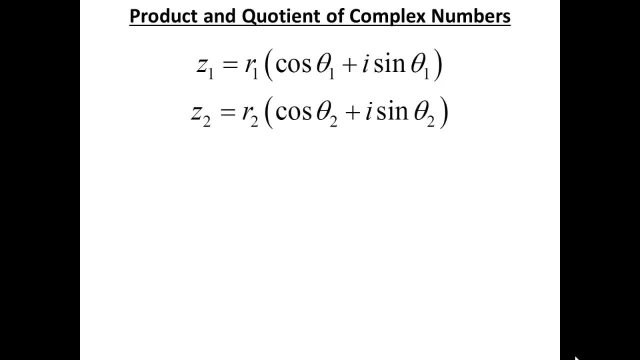 recognize the shortcut and then from this, that point forward, we can just always use the shortcut. So if I were to multiply these numbers together, I get this ugly looking thing right here where I have the first number times the second number. but I can realize this is really not the first number. 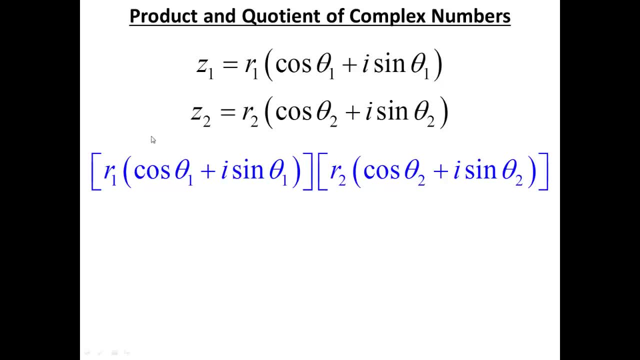 times the second number. these are four separate quantities being multiplied together. I've got r1. I've got the trig quantity here. I've got r2- I've got the trig quantity here. so those bracket parentheses I really don't need, because it's just four things being multiplied together. 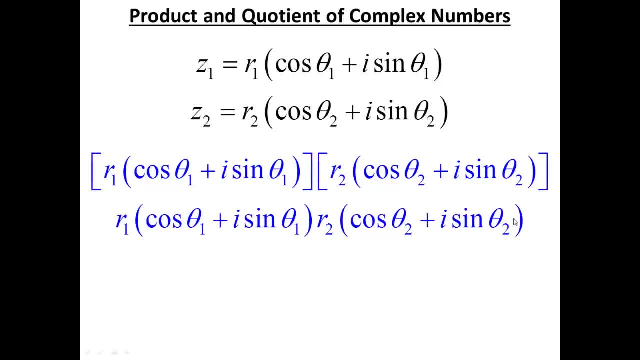 Now, first thing I'm going to do is I'm going to reorder the terms r1 and r2. I'll just go ahead and group those together and realize that r1 is just going to get multiplied times r2, and then for the rest of it I can just FOIL it out. So I'll take it moving to the top. 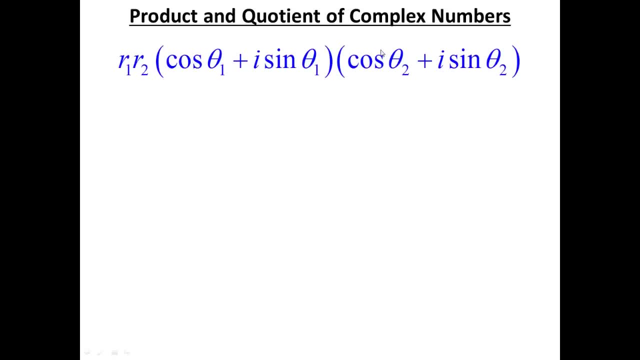 and then start FOILing it out, I'll know that this cosine gets multiplied by that times That cosine, and then cosine times this sine, and then this sine times that cosine, and then this sine times that sine, and it's going to come out looking like this and it may look like a lot until 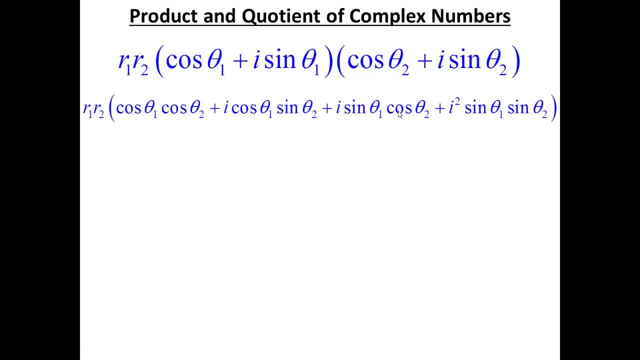 we realize that this can be simplified to something much prettier, much simpler. So we'll start with that: i squared. I squared is negative one, so that's going to be minus sine theta one, sine theta two. I'm also going to realize that the middle terms have i's, but the outside terms do not. 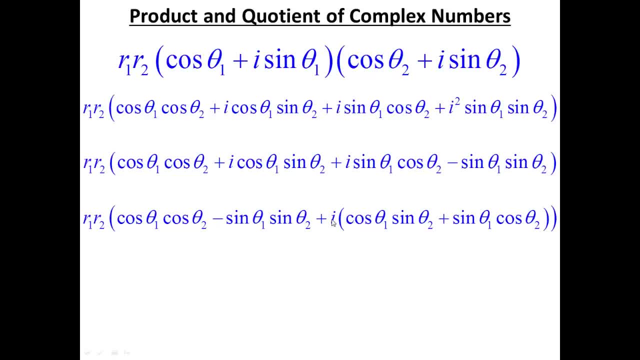 So I will go ahead and regroup those two terms together and factor out the i. So here are my non imaginary terms and here are my imaginary terms. Now, if you are really astute and you're really paying attention, you'll recognize something right here. 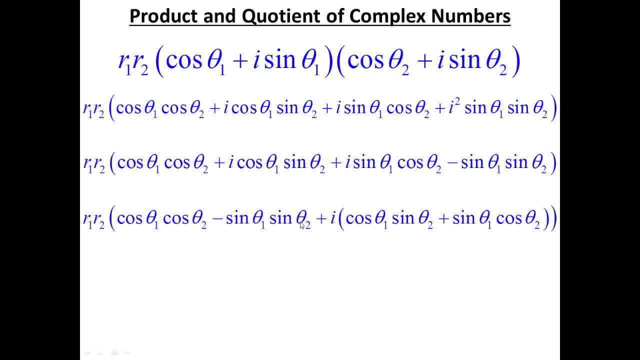 Cosine theta 1, cosine theta 2, minus sine theta 1 sine theta 2.. Hey, from chapter five, that's the cosine sum formula. Remember that, cosine. this is always going to be the opposite of what I was actually doing with the angles, Since, since this is minus one and this is, 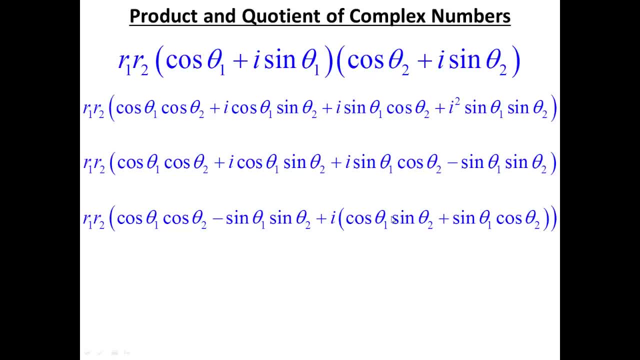 minus. that means this must be the cosine sum formula and, for that matter, when I mix and match the sines and cosines, that is the sine sum formula. so this could be turned into cosine of the sum of the angles theta 1 and theta 2, and this is sine of the sum of theta 1 and theta 2. so this is a 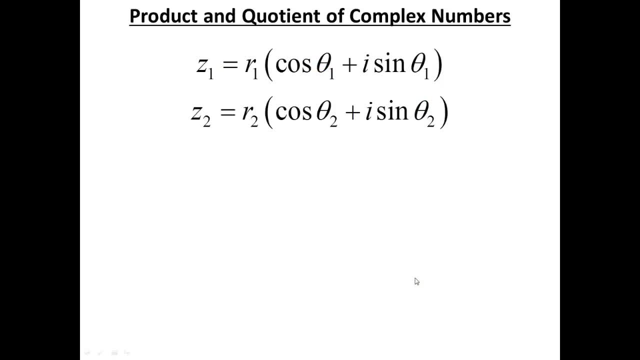 simplified version of foiling all that out. so in the future, instead of trying to multiply these through and foiling it all out, I can just realize that if I want to multiply z1 and z2, start by multiplying the radii r1 and r2 and just add the angles together. don't waste time foiling anything. 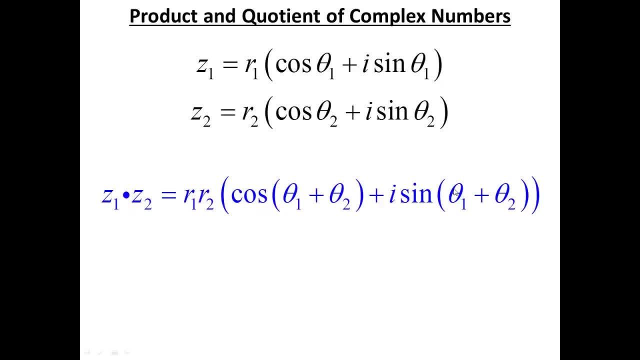 out. just add the angles together, once for cosine and once for sine, and if I know that's true, I can make the logical leap to division: that instead of multiplying the r's and adding the angles, I will divide the r's and subtract the angles. so from this point forward, multiplying and dividing complex. 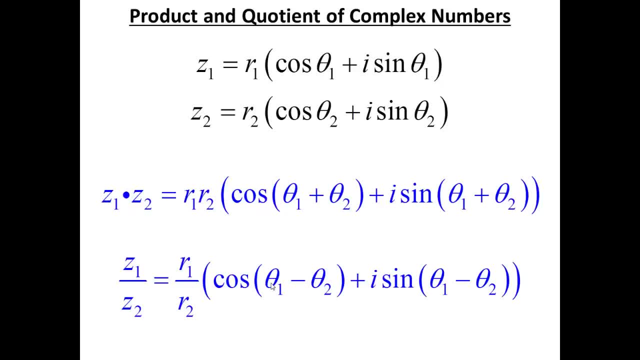 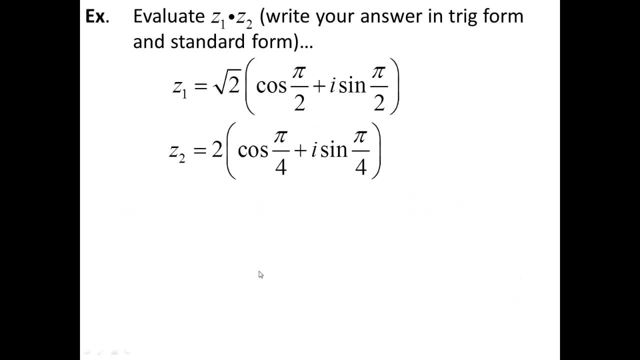 numbers in trig form is just a matter of either multiplying or dividing the radii, adding and subtracting the angles. so let's look at an example. so let's start by taking these two complex numbers currently written in trig form, multiply them together and then we will simplify it down to standard form. so we will start. 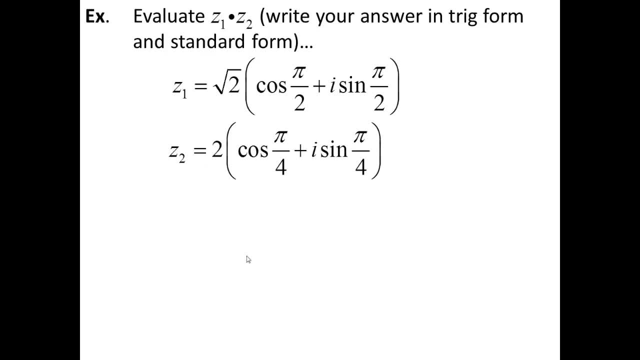 by multiplying the radii root 2 times 2 is just 2 root 2, and then we're going to add the angles together: pi over 2 plus pi over 4. now to add it together we need a common denominator. so pi over 2 plus pi over 4 is going to have a common denominator of 4. pi over 2 is really 2 pi over 4. so 2 pi over 4 plus 1 pi over 4 would end up being 3 pi over 4. so here is my answer in trig form, but we also need to take my answer and write it in standard form, and that's easy enough. all we have to do is simplify it down to standard form by evaluating the cosine and the sine. so cosine of 3 pi over 4- that's going to be negative root 2 pi over 4 plus pi over 4 is going to have a common denominator of 4. pi over 2 is really 2 pi over 4. so 2 pi over 4 plus 1 pi over 4 would end up being 3 pi over 4. so here is my answer in trig form, but we also need to take my answer and write it in standard form, and that's easy enough. all we have to do is simplify it down to standard form by evaluating the cosine and the sine. so cosine of 3 pi over 4, that's going to be negative root 2 pi over 4 plus pi over 4 is going to have a common denominator of: 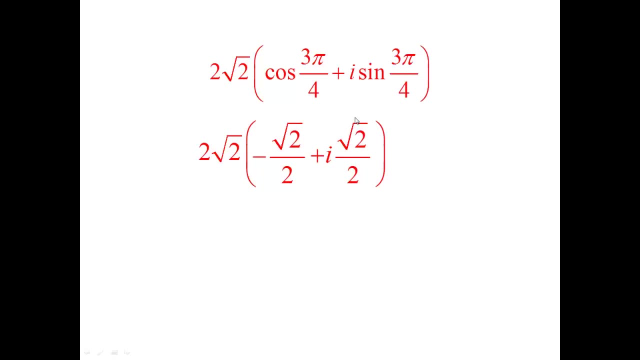 2 over 2, sine of 3, pi over 4, positive root 2 over 2. now, technically right here, this is acceptable as a standard form of an angle. it kind of depends on what the numbers look like as to whether I'm going to distribute that to root 2. on the outside this one numbers look pretty simple, pretty reasonable, so I'll go ahead and make that extra step. when I distribute the 2 across, it's actually going to cancel with both of these 2's on the bottom, so all of the 2's are going to cancel out. and then when I distribute the root 2, 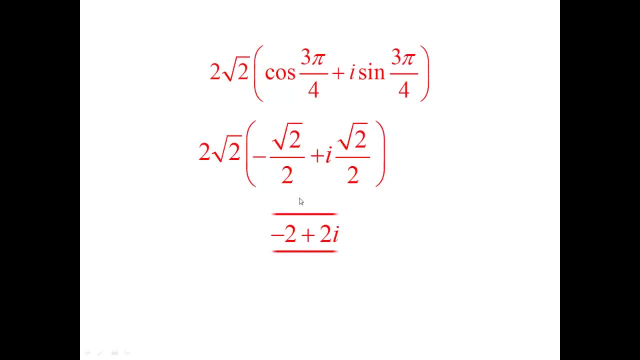 well, root 2 times root 2 is just 2 itself. so that means it's going to simplify to negative 2 plus 2i. so trig form, standard form. alright, here is another one. why don't you try this one on your own? this time we are going to divide, so we're still going to follow the same basic technique and notice, it's the same numbers that I used before. give it a try, hit, play when you're ready. alright. so when we divide, we divide the radii. 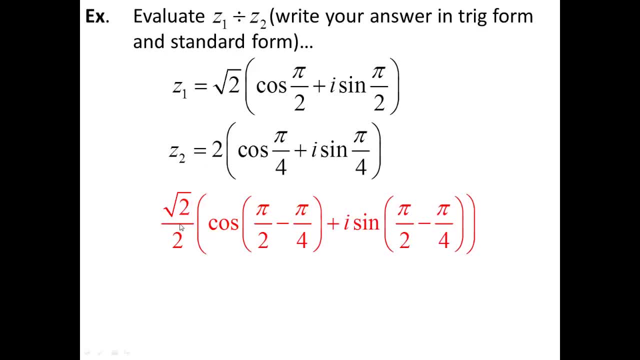 and subtract the angles. so root 2 divided by 2 would be on the outside, and then pi over 2 minus pi over 4 on the inside. remember that this was 2pi over 4. so 2pi over 4 minus 1pi over 4 would just be 1pi over 4. so there's my trig form. 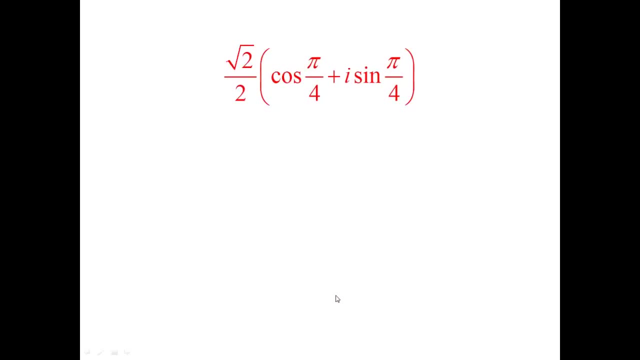 simplify to get my standard form: cosine and sine of pi over 4 are both root 2 over 2. if I distribute the root 2 over 2 on the outside root 2 over 2 times root 2 over 2, it's just going to be 2 over 4. 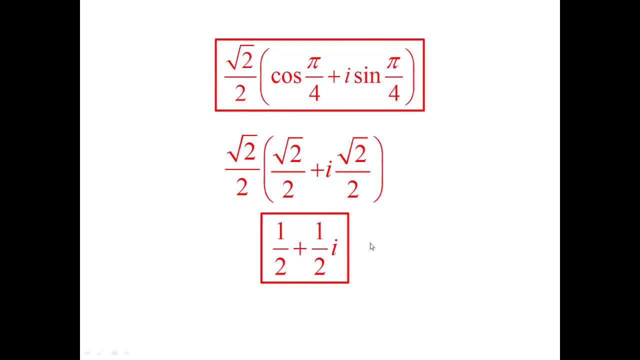 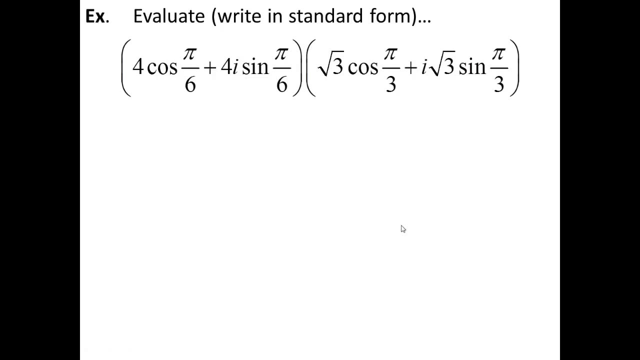 which is really one half. so one half plus one half I all right, here's another one. once you give this one a try, hit play when you're ready. all right, first thing I want to do is recognize what the radii is for each of these guys on this. 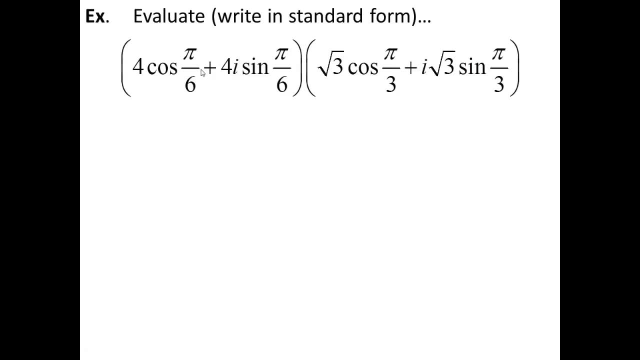 one notice the it's. it is trig form it just have- has the radii radius distributed through. so the radius over here would be 4 and the radius over here would be root 3. so 4 times root 3 would be 4 root 3 and then, if I take the, 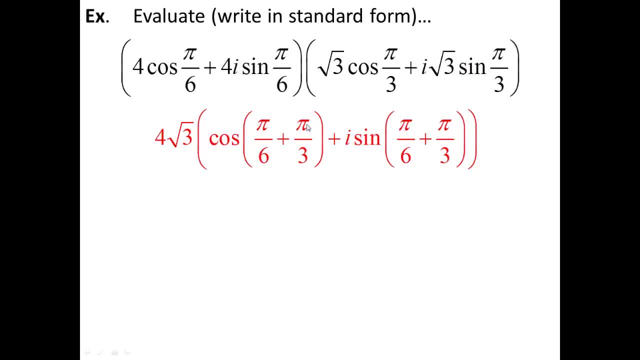 angles and add them up: pi over 6 plus pi over 3. keep in mind that pi over 3 is really 2, pi over 6, so I would end up with 3 pi over 6, which is really pi over 2. cosine of pi over 2 is 0. sine of pi over 2 is 1, 0 plus I is just I, so my 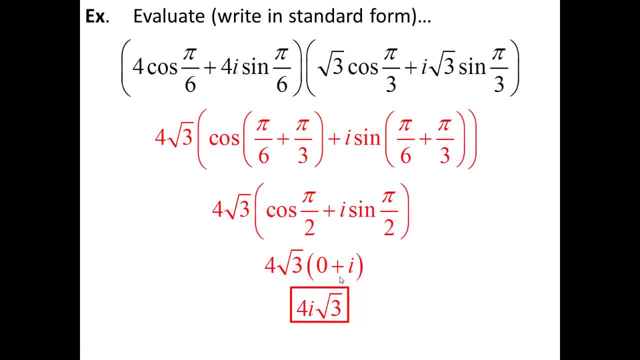 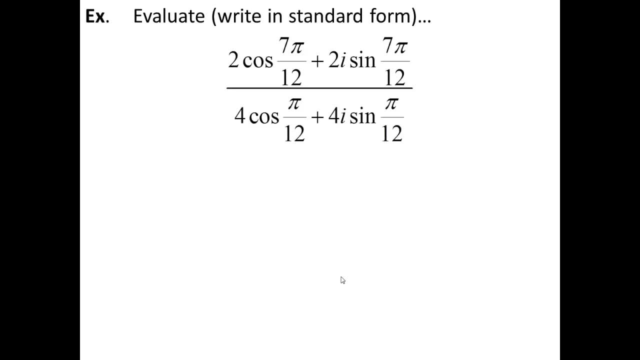 final answer would be: 4i root 3. all right, do it one more time, this time different. divide. hit play when you're ready, all right. so radius of 2, radius of 4. if I divide I would get 1 half and we will subtract the angles 7 pi over 12 minus. 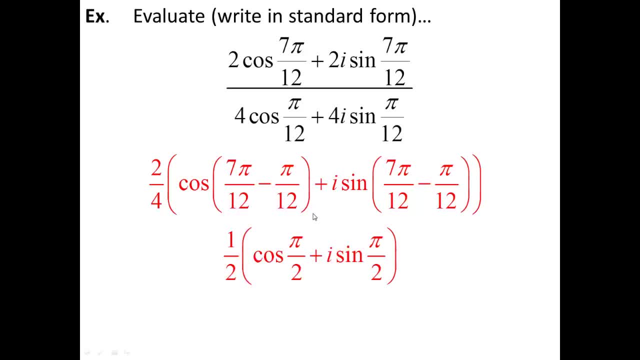 pi over 12, that would just be 6 pi over 12, which is really pi over 2. cosine of pi over 2 is still 0, sine of pi over 2 is still 1, 0 plus. I is still just I, so my. 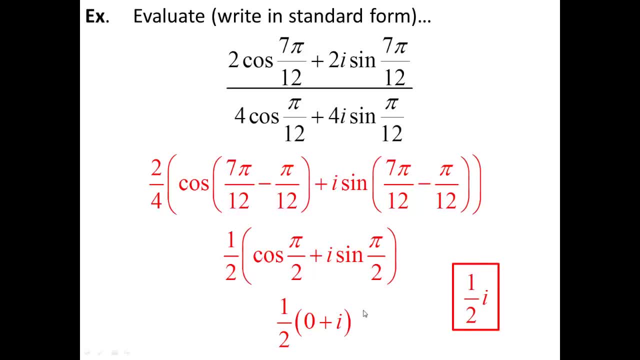 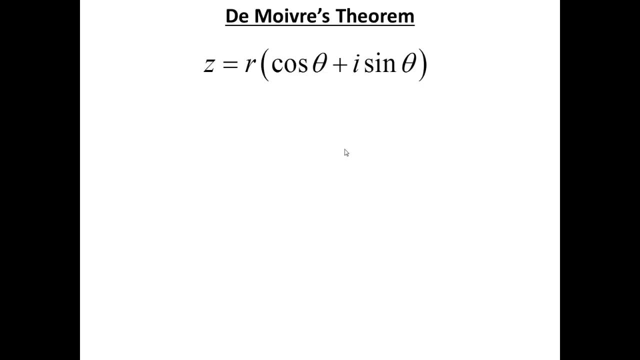 final answer would be 1 half I, and so we finally come to DeMoise theorem. we've done all this prep work just to get to these final few bits on DeMoise theorem. now we learned about complex numbers, we learned how to write them in standard and trig form, and then we learned how to 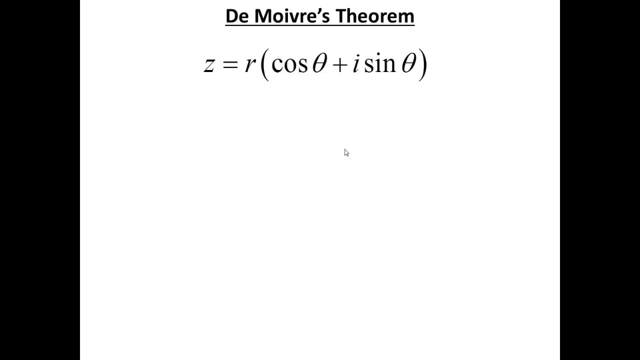 take trig form and multiply or divide different types of trig form numbers. now let's do DeMoise theorem. let's figure out what DeMoise figured out on his own. so imagine I take a complex number written in trig form: r, cosine, theta plus i, sine. 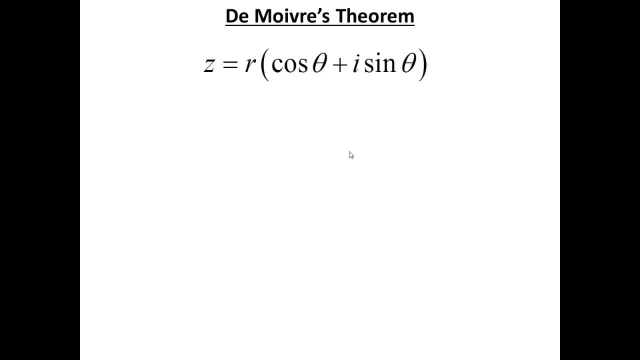 theta and I want to multiply it times itself. well, of course, multiplying times itself, that's just another way of saying squaring it. now, if I'm taking r cosine theta plus i sine theta and multiplying it times r cosine theta plus i sine theta, well, r times r is going to. 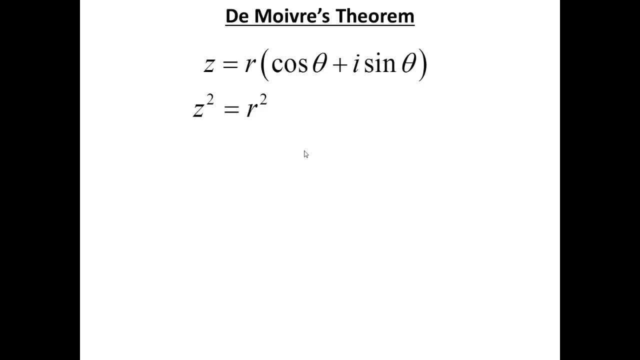 give us r squared and then with the angles we add them together. so if I take the theta from this one and then the theta from this one again and add it together, I would just get 2 theta. so when I multiply it times itself when I square it. really I'm just going to square the r and I'm going to double the angle. 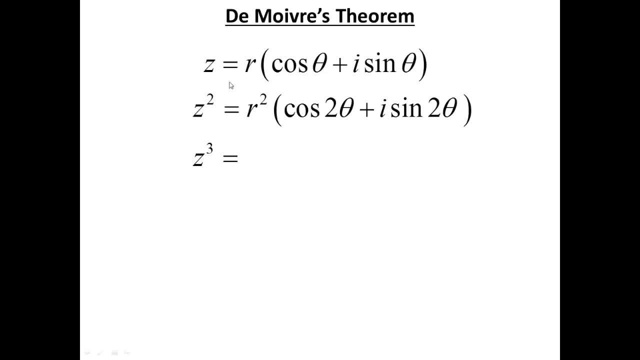 and for that matter, what if I wanted to cube it? well, cubing it is really just taking the square and multiplying it times the original, because of course z cubed is just z squared times z. so if I take r and multiply it times r squared I. 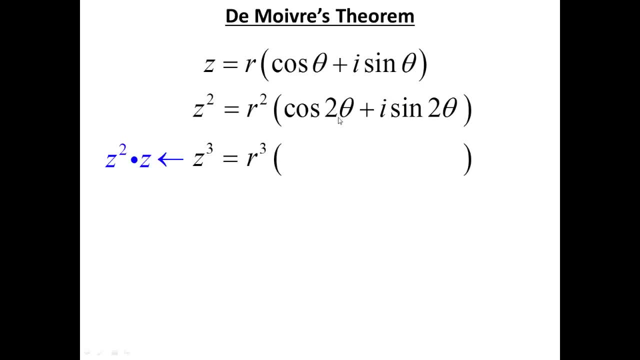 would get r cubed. if I take theta and add it to 2 theta, I would get 3 theta. so hopefully we're starting to notice a pattern here. if I want to take a complex number written in trig form and raise it to any power, it's just a matter of. 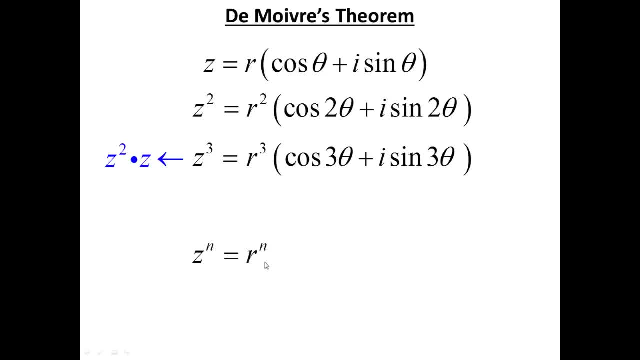 starting with the radius and raising it to v and then raising it to the nth power. if n equals 50, then I'll raise it to the 50th power, and then, with the angle, we don't raise the angle, we multiply the angle times, whatever that. 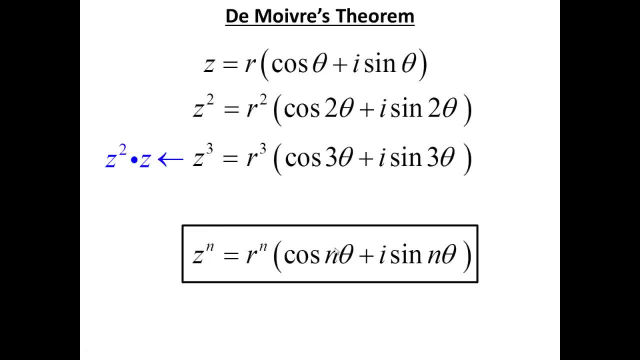 n value is, and there is de Moise's theorem. instead of taking the standard form of a complex number, let's say 1 plus 2i, and raising it to the 50th, in which case we would have to write it out 50 times, foil it out, multiply it through, distribute and. 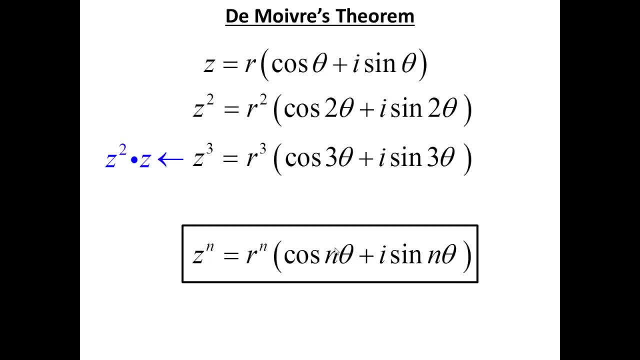 it would take forever and a day to do all that arithmetic. if it's in complex form, it's going to be much, much quicker. it's just a matter of taking the single number r, raising it to the 50th power, and then taking theta and multiplying it times 50 and simplifying. 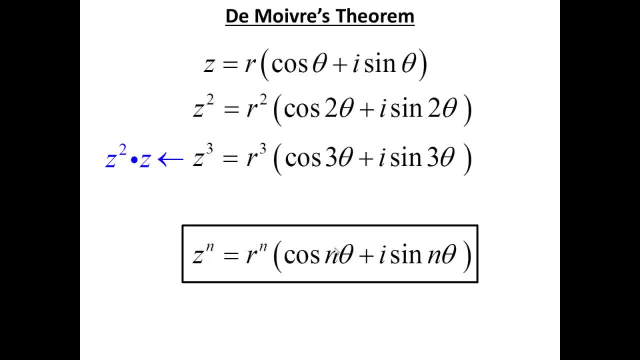 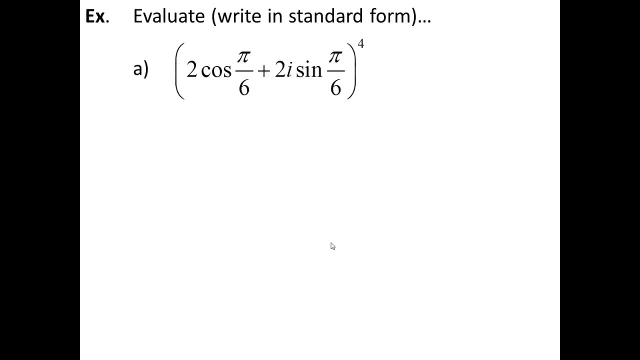 from there. it's much quicker and easier when you are in trig form to raise it to absurdly large numbers, versus when it's in standard form, raising it to absurdly large numbers. for example, let's look at this number raised to the fourth power. we're going to write our final answer in standard form now, if this we're already. 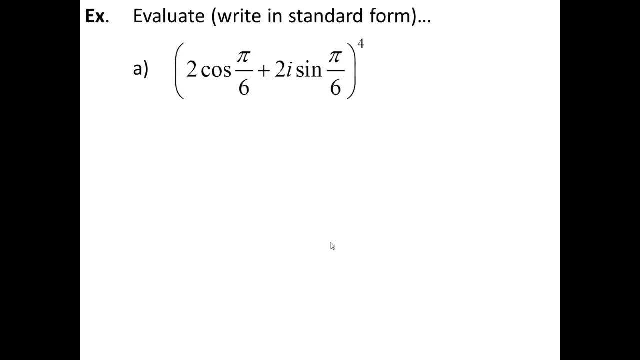 in standard form and I wanted to raise it to the fourth power. I would have to write it out four times and FOIL it out, and it would probably take half a page to complete. Likewise, I could do the same thing on this one. It is a binomial and I could. 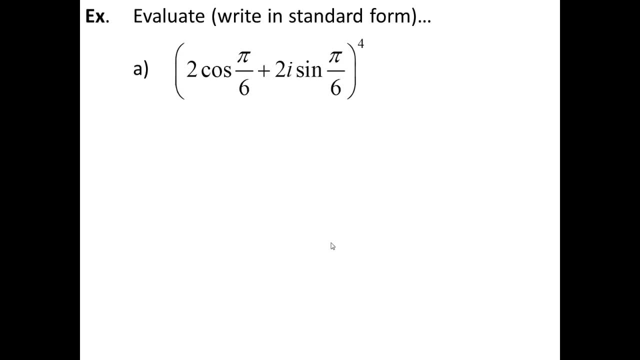 write it out four times and FOIL it all out and simplify it, and it would take me half a page to get through it. Or I can remember DeMoine's theorem. DeMoine's theorem says: simply take the radius, in this case, which is 2,. 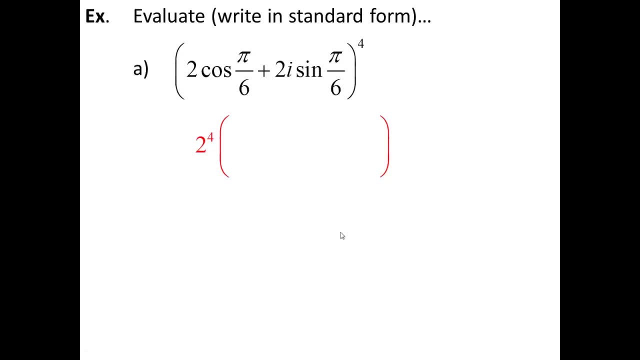 raise that to the fourth power and then take the angle pi over 6 and multiply it times 4.. From here it's just a matter of simplifying. So 4 pi over 6 is really 2 pi over 3.. 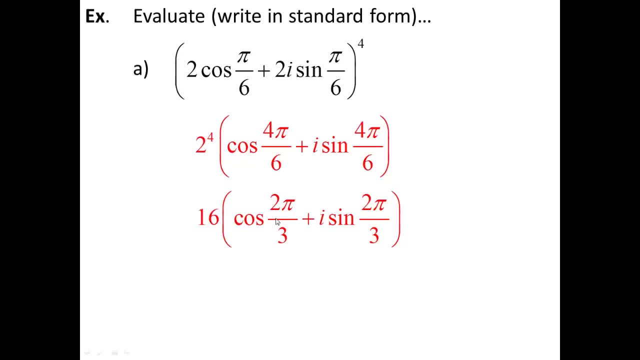 2 to the fourth, of course, is 16.. Cosine of 2 pi over 3, that's going to be negative, I'm sorry, yeah, negative. one half Sine of 2 pi over 3 is going to be root 3 over 2.. Distribute the 16.. 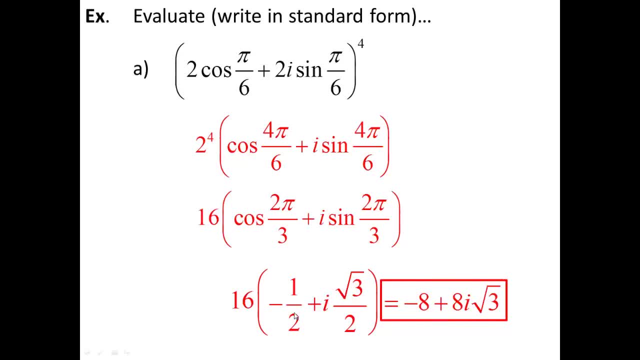 Well, the 16 is going to cancel with the 2, so I'm going to get negative 8 plus 8i, root 3. And I would be able to do that in just a couple of lines of space instead of taking the half page. 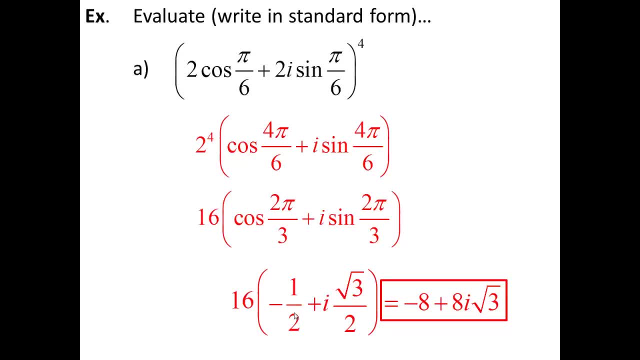 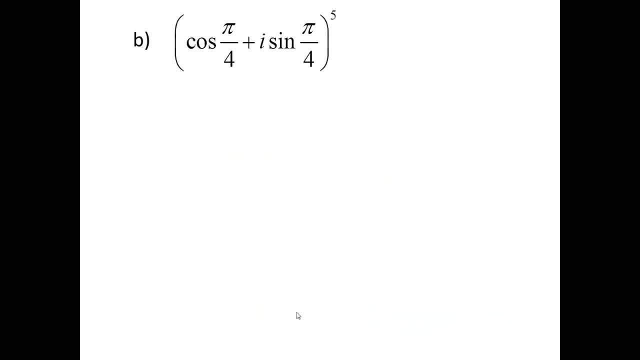 I would need to FOIL all of it out. Much easier to use DeMoine's theorem than to actually expand out the binomial. Alright, here's another one for you to try on your own Hit play when you're ready. Alright, first thing, I'll recognize. 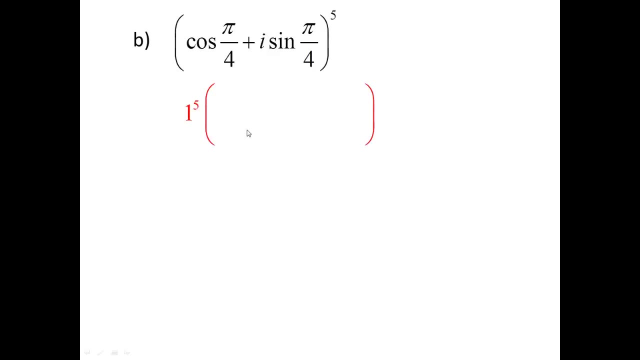 is what the r-value is. Since I don't see anything, the r-value must be 1, so I'll raise 1 to the fifth and then I'll multiply pi over 4 times 5.. 1 to the fifth, obviously, is still going to be 1, so I can ignore that from this point forward. 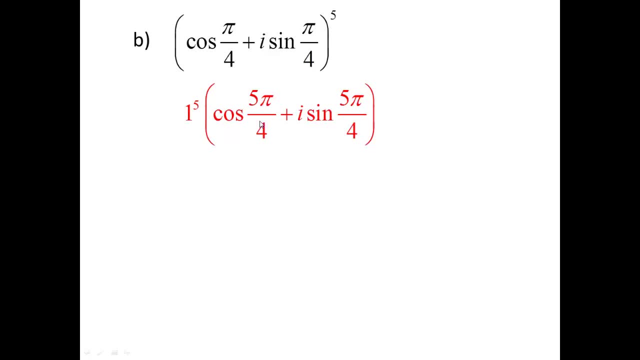 Let's just evaluate the inside Cosine of 5 pi over 4,, third quadrant. negative root 2 over 2.. Sine of 5 pi over 4, still in the third quadrant. so negative root 2 over 2.. 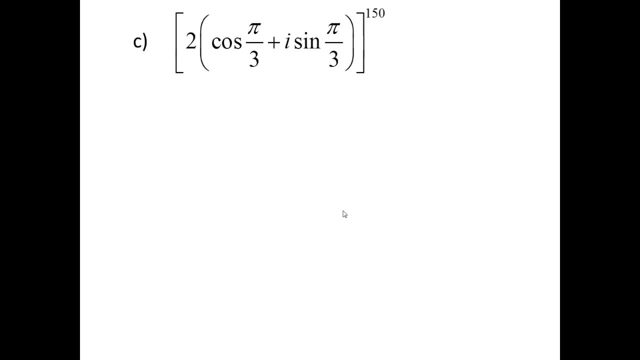 Final answer. Here's another one. Try this one out for size. Alright, so here is where DeMoine's theorem really shines. I've got it raised to the 150th power. There is no way I would ever attempt to do this. 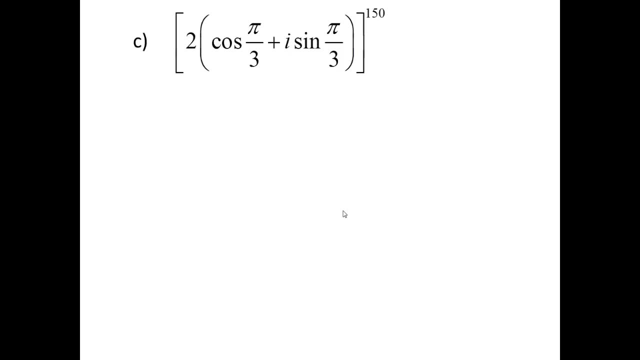 by just FOILing everything out. As soon as I saw 150th power, I would just say: screw it. I'm not even going to try this one. I'll lose the point. I'm not going to waste time doing all this. I'll move on to. 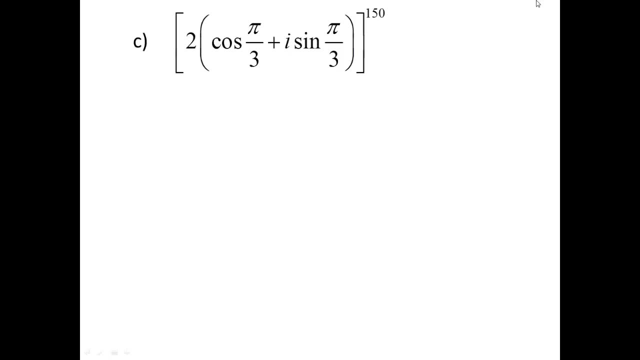 something easier, But with DeMoine it is pretty easy. I'm going to raise 2 to the 150th power. Now that, right there, that's not something I would be able to evaluate. simply, It's not something I would. 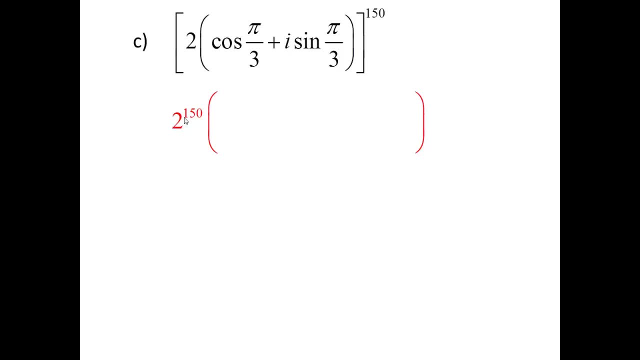 even really be able to evaluate with a calculator. Most likely, if I type that in a calculator it would give me an overflow error. So this is a situation 2 to the 150th. I am not going to simplify that at all. I'm going to leave that as 2 to the 150th throughout the problem. 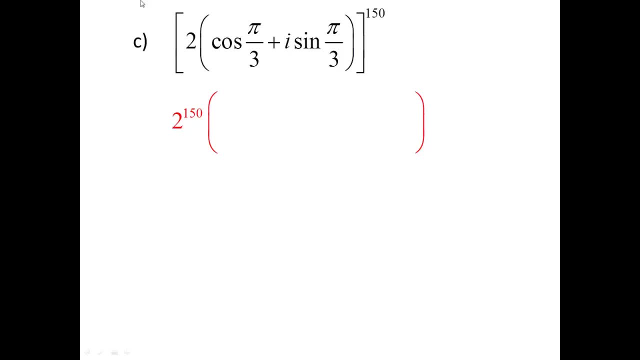 My final answer will have that: 2 to the 150th in the problem. Now for the pi over 3, when I multiply it times 150, that seems like oh my gosh, that's such a large number. until I realize that 150 divided by 3 is just 50. And 50 pi is. 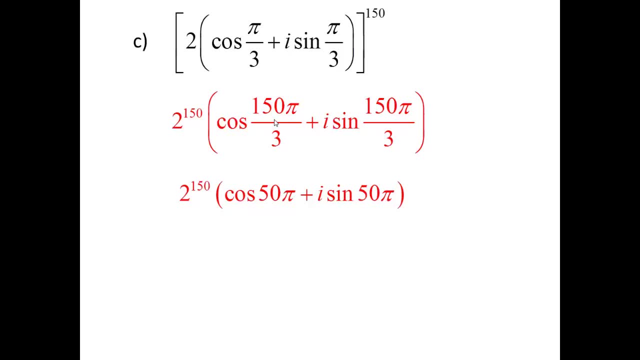 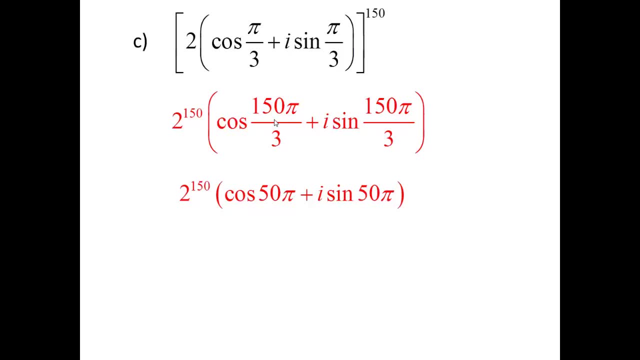 0.. 6 pi, I'm back to 0.. Any even pi, I'm going to be coterminal to 0. So I can really think of that as cosine of 0, sine of 0, cosine would be 1,. 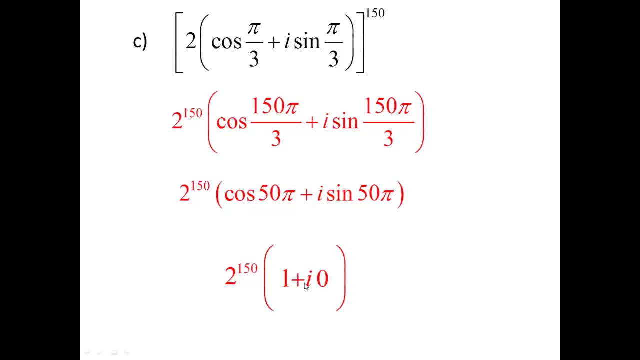 sine would be 0. So this is really just 1 plus 0, which is 1, which means my final answer is 2 to the 150th power. How pretty is that? Alright, here's another one: 3 plus 4i to the 20th. Now, first thing I'm going to notice is that this: 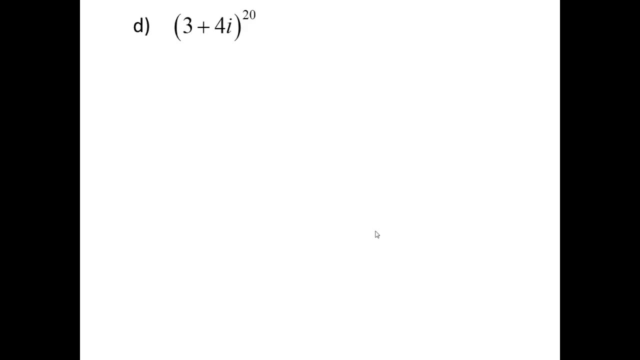 one looks a little bit different. It's in standard form, raised to the 20th, instead of trig form, raised to the 20th. And no, I do not want you to write this out 20 times and multiply it through If it's not in the 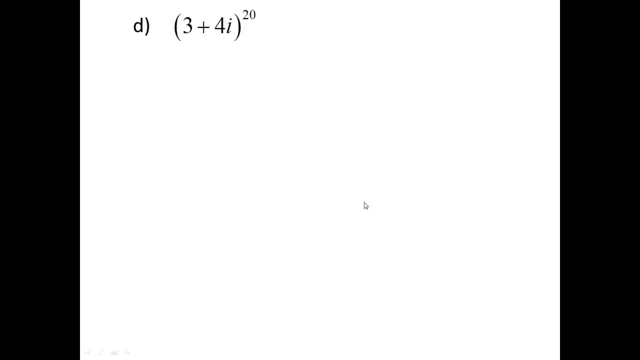 appropriate form to multiply through. let's go ahead and put it in the appropriate form. Let's start by converting 3 plus 4i into trig form and then we can apply DeMois's theorem, So 3 plus 4i into 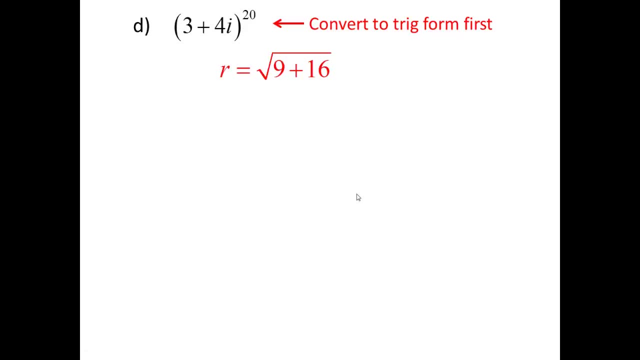 trig form. So we'll start with the radius a squared plus b squared, 3, 4 is really just going to be 5.. And then to get the angle we'll do inverse tangent of 4 over 3.. We're in the first quadrant, so no adjustment is necessary. I'll pull out. 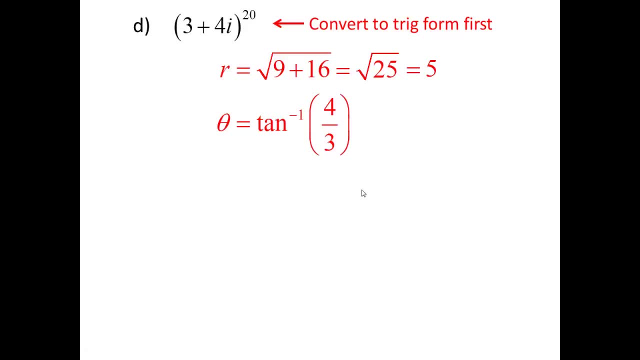 my calculator. Now, it really doesn't matter whether you do this in radians or degrees, because the angle is not going to be a part of my final answer. I'm going to figure out what the angle is, either in radians or degrees, But then as part of my 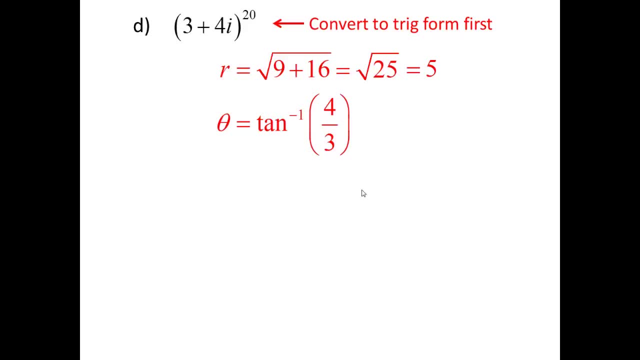 final step. I'm going to evaluate at that angle, So there's really no need to worry about whether your degrees or radians just remain consistent. So, quadrant 1, I am going to stick with radians because I like radians more than degrees 0.927.. And if you were working? 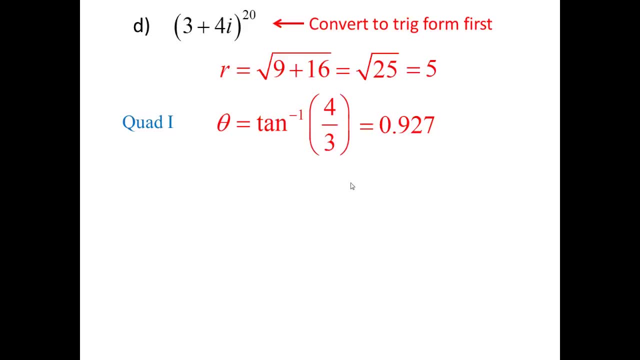 in degrees, you should be getting 53.130 degrees, but I'm going to stick with radians. So I'm going to take my radius and I'm going to take my angle- 0.927, and rewrite it in trig form. 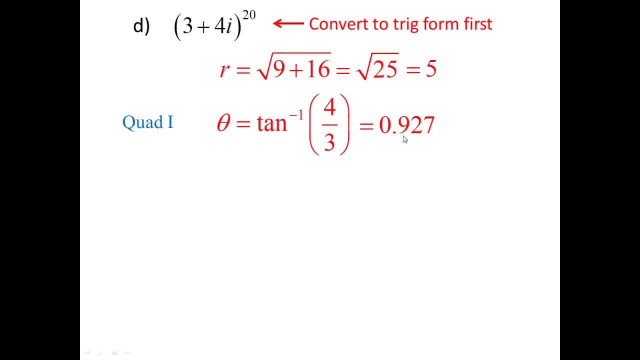 Now I know I'm going to be using this number several times over and over again in this problem. So before I do anything, I will go ahead and store that in my calculator and I'm going to store it for a. And now, by doing: 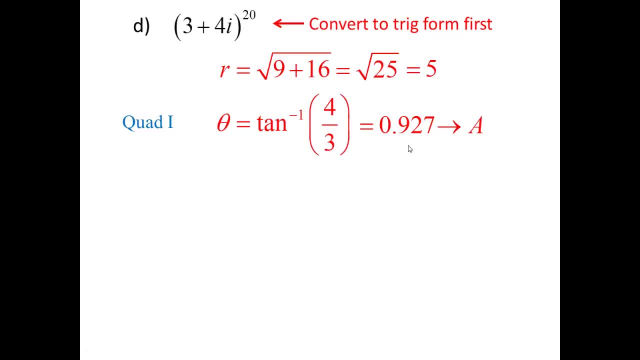 that, and by writing it down I actually don't ever have to write down the 0.927 again. I can just write my angle as a, because my calculator knows what I mean. So here's my trig form raised to the 20th power. Now I can do. 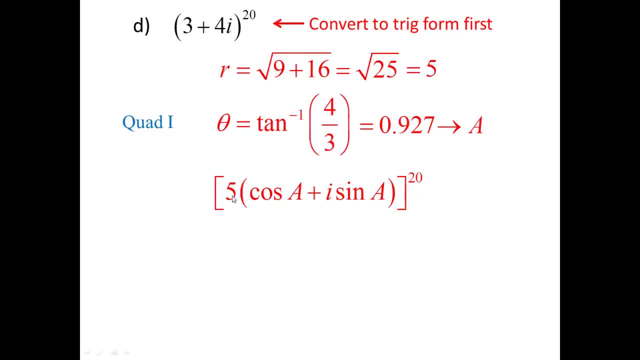 just like I did on the last few problems, Start with the 5, raise it to the 20th and then take the a multiply it times 20.. So from here I can just evaluate Now 5 to the 20th. 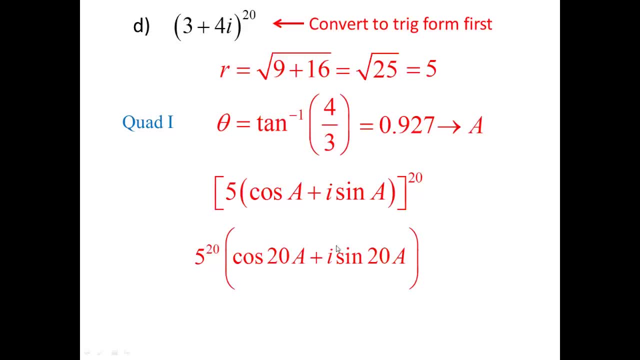 that is an insanely large number, so I'm not going to worry about it. I'm just going to evaluate the inside As soon as I evaluate the cosine and the sine, as soon as there is no longer a cosine and a sine in the problem. 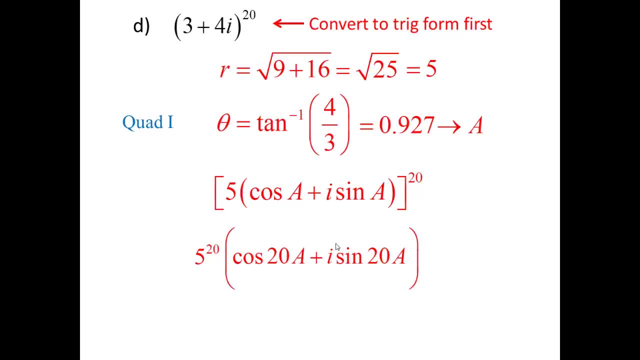 I am then in standard form, even if I don't distribute the 5 to the 20th. So when I evaluate each of those, I get 0.954 and 0.299.. So this is what I'm going to call my final answer.